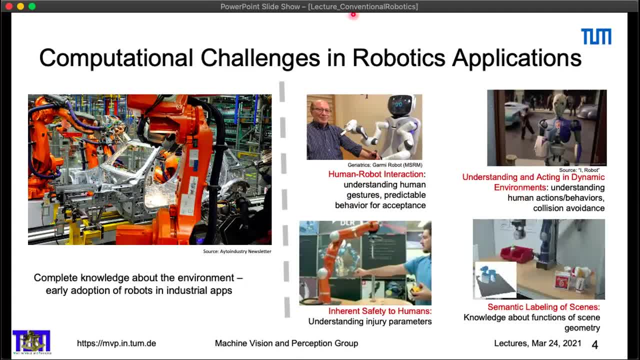 I want to understand. Let me just move me to. I want to understand basically what actions are happening, so interact with dynamic environments And I would like to also have a safe interaction. So one of my former PhD students, a professor at TUM, actually started the field of safety and robotics work. 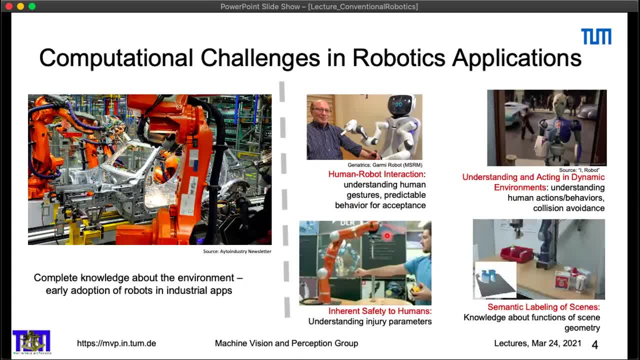 His famous video was really. he took a disc and let the robot hit His hat with a disc just to prove that he can safely interact with the robot. This was pretty scary but got him a professorship And something you may be used to actually also understand what's in the scene. 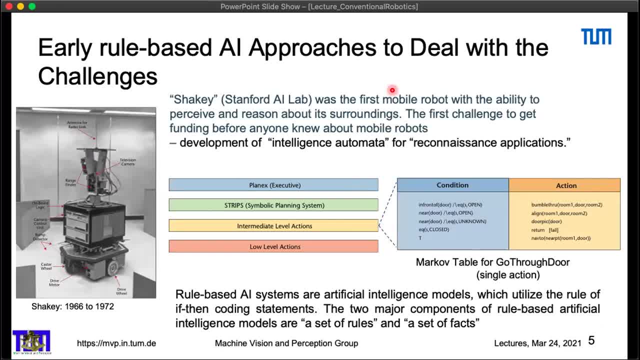 So it's a little bit of an AI. so you will be surprised, but AI goes back all the way to 72,. you may know the shaky robot at Stanford. you still see him in the entrance to the computer science building And back then people. 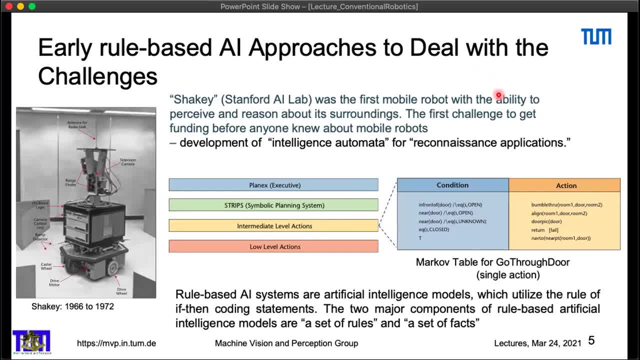 were working on rule-based AI, so they tried to actually find a set of rules- how to actually interact with the environment, And what they developed back then is still something we use on the robots these days. so we have this hierarchy from low level processing all the way to planning. 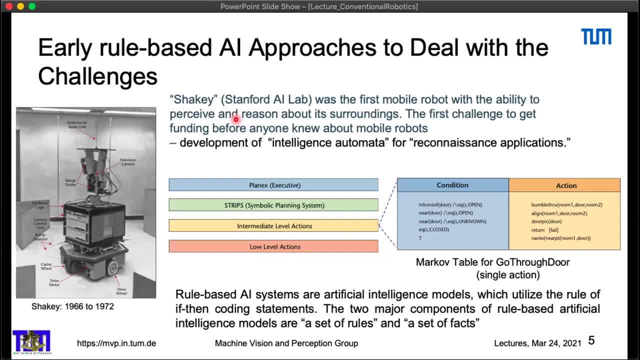 And the problem they were having back then is actually nobody knew what a mobile robot is, so it was really a challenge to apply for the funding. so they applied back then for development of intelligent automata, For reconnaissance automata, applications, just because nobody at the funding agency had any clue about what a mobile robot is. 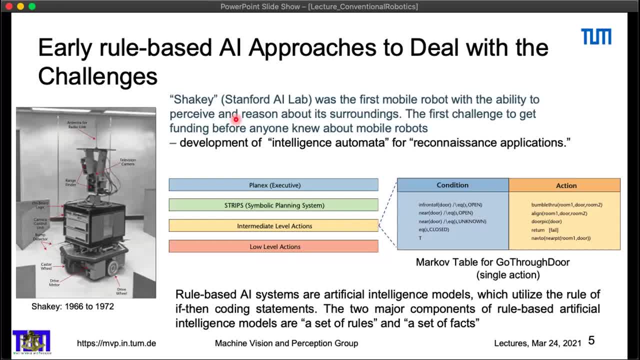 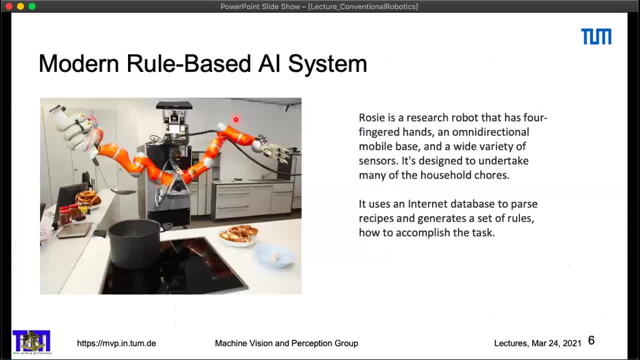 So what they were trying to really develop and what people worked on for quite a while were rule-based AI systems. And another example, now a more recent one, is, for example: well, this robot looks pretty funny. maybe it's Rosie. it's a robot developed here at TUM, now moved to Bremen. it's the robot which uses basically. 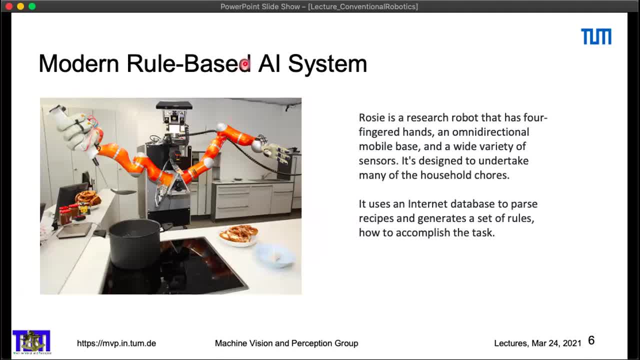 rules which are read on the Internet. so it goes on, the web browser gets a recipe of something to cook and it's cooking it basically in the kitchen, just by following recipe which is downloaded from the web. so the rule is really something which comes from the web and the robot just repeats it. 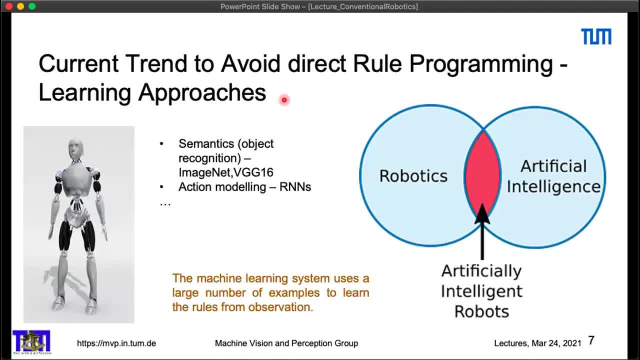 it's, of course, very tedious to build all the rules. maybe that you can use Google, but the current trend, as you all know, is that you can use Google, But the current trend, as you all know, is that you can use Google, But the current trend, as you all know, is that 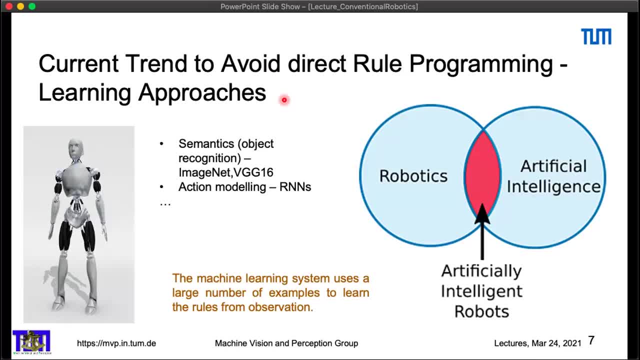 you would like to avoid the programming and would like to have the robot learn it by itself, and the current approaches basically go towards semantics- understanding what's in the scenes, object recognition, object labeling- and the other challenge is basically action modeling, something like RNNs. 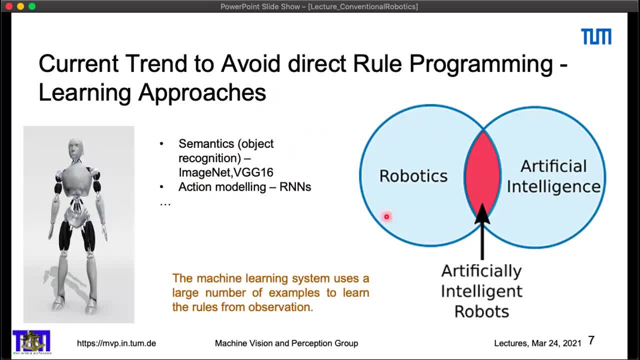 But if you look at robotics, there is this huge field of robots, most of them in the industry, these blind robots repeating the task, And there is a huge field of artificial intelligence, and the intersection where the robots actually use the intelligence for the task is very small. so this will be the 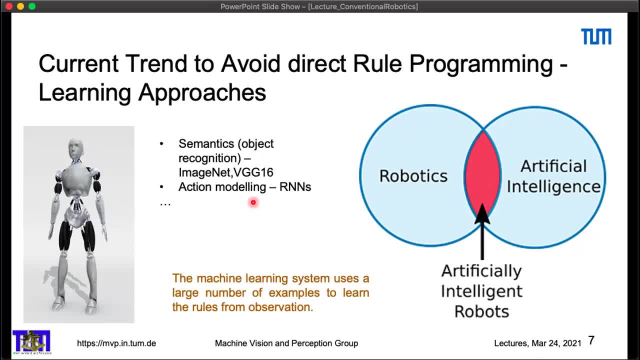 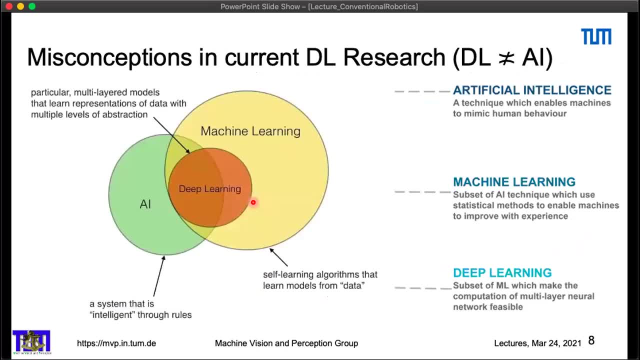 Artificially intelligent robot, robots which actually respond To the environment. What I'm fighting for quite a while- I think Ioanna will know the pain- is that people have started calling a deep learning AI, Which is not really true. If you look at the things is basically AI is a huge field, what deep learning is really a small subset of, and there are intersection fields between AI- deep learning- and AI- machine learning. because, if you think, 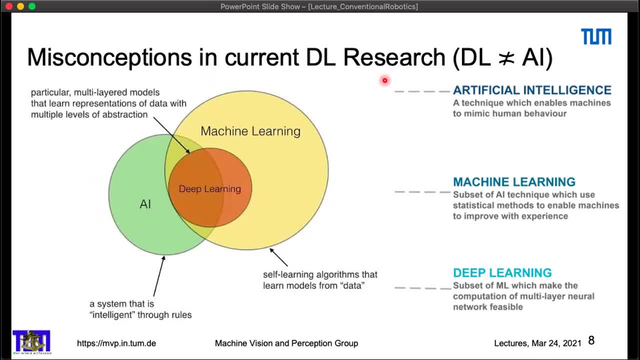 About AI. it's a technique which enables machines to mimic human behavior. it's not set if it's derived from data. if it's, if it's rule based or whatever way you want to call it, It's going. and then there's a subset of machine learning, which is a subset of AI techniques which use statistical methods to enable machines to improve. 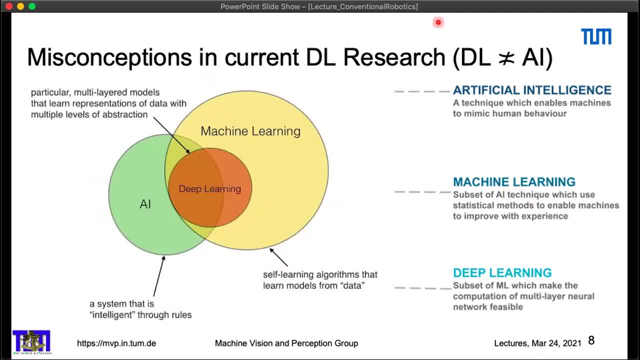 Experience. again, it's not necessarily said that this data driven. and then there is this deep learning, which most of you, I guess, these days, are interested in. so i'm always kind of wondering why everyone said he works on AI, but in the end he's working on deep learning. 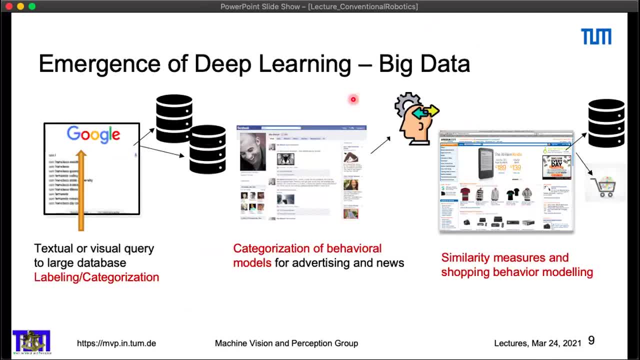 Where does it come from? so, basically, I think deep learning emerged from the necessity to do these three tasks: to label and categorize things. this is what Google was interested in, if they have this huge data database in which they wanted to provide fast access to. so they were interested in categorization and fast access to the response. 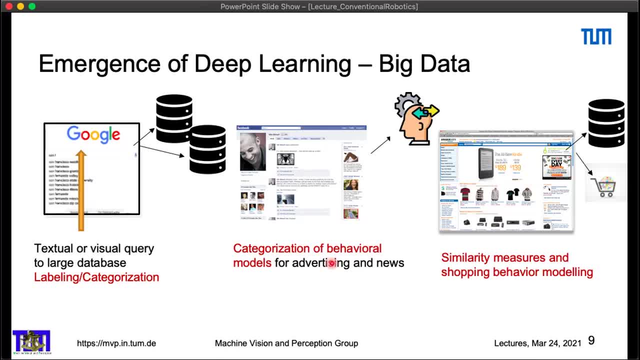 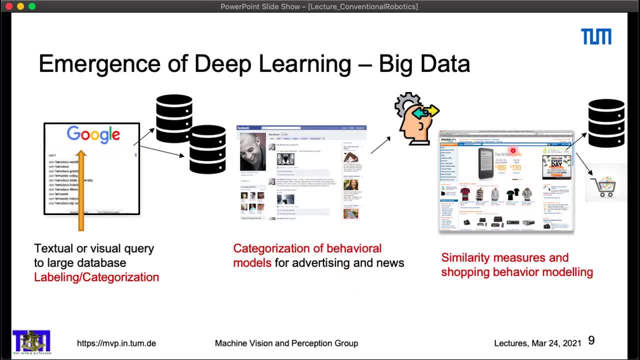 To get physically, To provide similar article to the one you're just looking at, and to Learn about your shopping habits. well, all these three have in common. common, basically, is they are really just used to Excellent the data- huge amount of data- and to find similarities between what's currently. 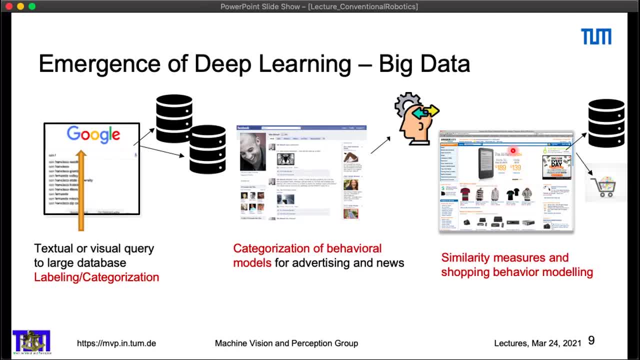 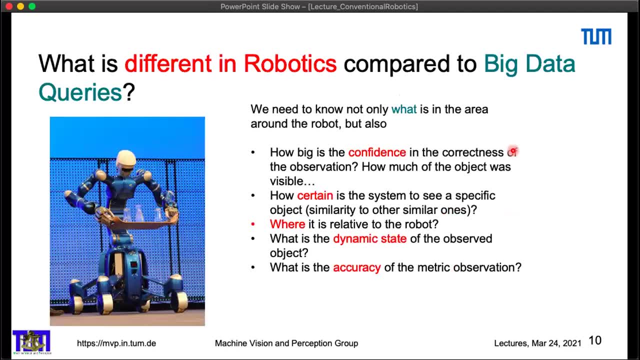 in front of the system and what's in the background? knowledge. now people try to use it in robotics, but now many of them forget that there is more than this which is required from an ai system. so what's different in robotics to these big data applications which? 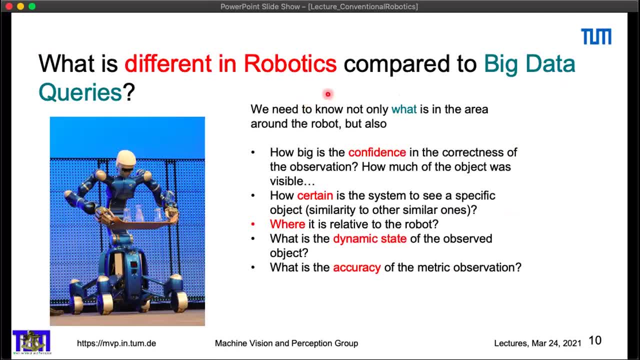 has looked at before. it's: basically we need not only to know what's in the environment- this is something your deep learning system can help you with- but we need to know a little bit more. the first important thing, which actually right now i'm working with multiple people, actually kind of- 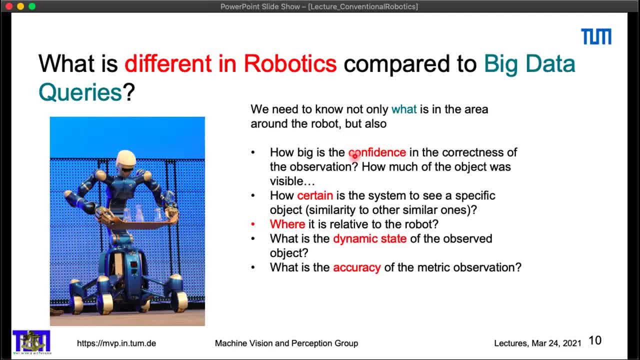 motivate the community to work more on this is to provide a confidence value to response. so basically, i'm not only interested to say it's a cup, but i would like to understand how much of the cup the system actually could validate in the image it could be. 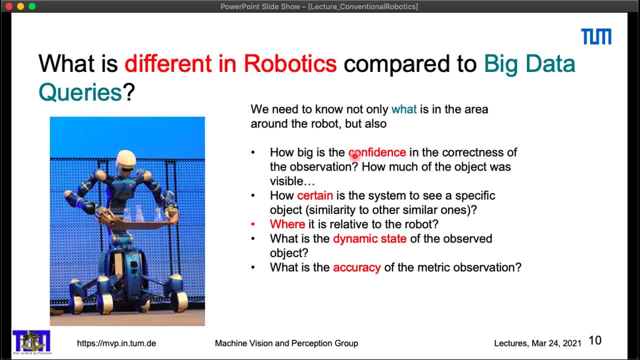 that it was seeing just a small corner of the cup somewhere and it's claiming there is a cup. so the confidence value would be very important for robotics. the certainty like how certain is the response? what you usually get from the network is basically a labeling: this is a cup, but you have no. 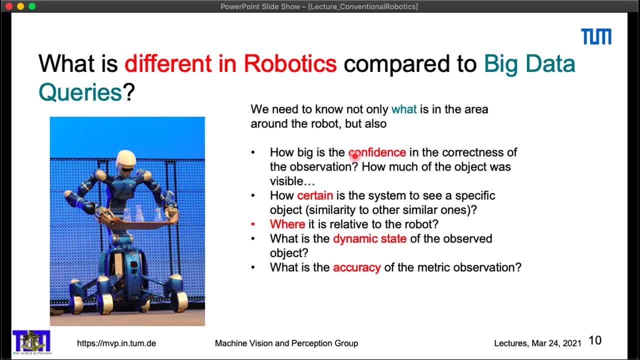 clue that there may be a different object which is very close to the response and that the system just kind of through the dices to decide cup and not mark or whatever. so certainty, and what the systems- current systems- are not doing is basically providing information where it is in the world. 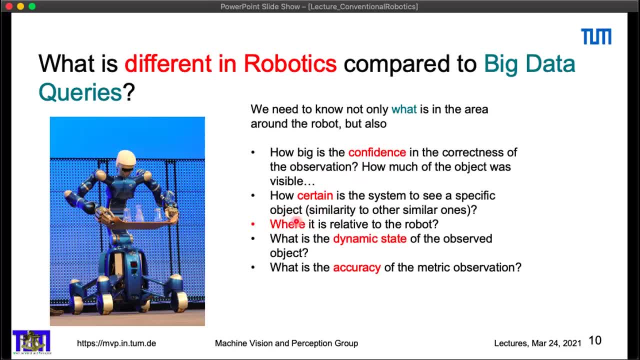 you know where is it in the image, but you don't understand basically the 3d position and you don't understand the accuracy. why is it important? i'm always saying, if you have a 95 system, so people always claiming you have a 95 to 96 percent accurate system in deep learning. 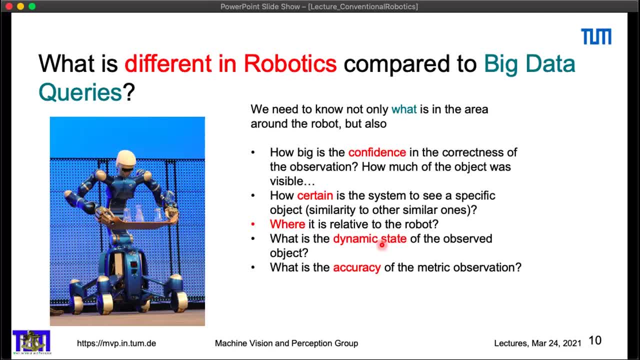 networks. this just means that if you run the robot 24 hours a day, then 72 minutes the robot has no clue what it's doing, and if you don't provide the measurements i just mentioned here, then the system will just go wild and the controller in the robot would not even know. 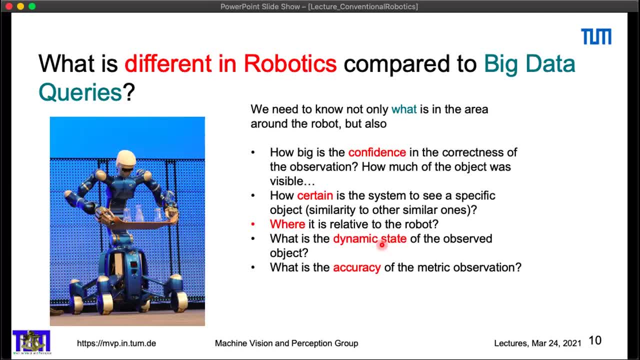 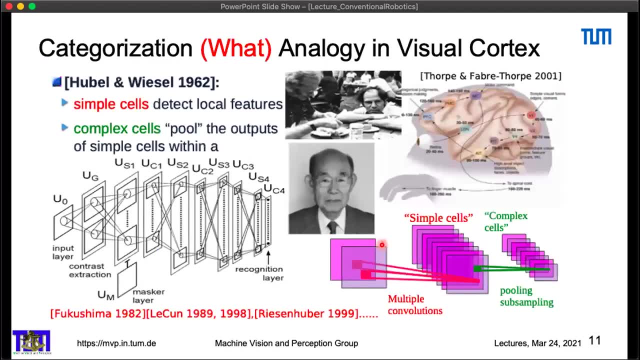 that something goes wrong. so providing these additional values is very important if you want to use it, not for labeling your pictures, but want to use it to control and make decisions. so we know that people are always motivated. the motivating that the deep learning nets kind of have an analogy to visual context. this is a slide from leon lecun, actually it's. 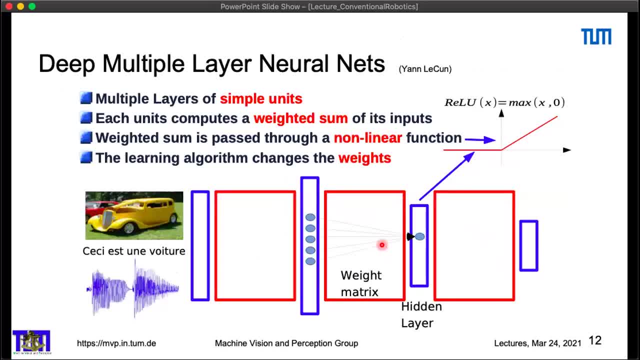 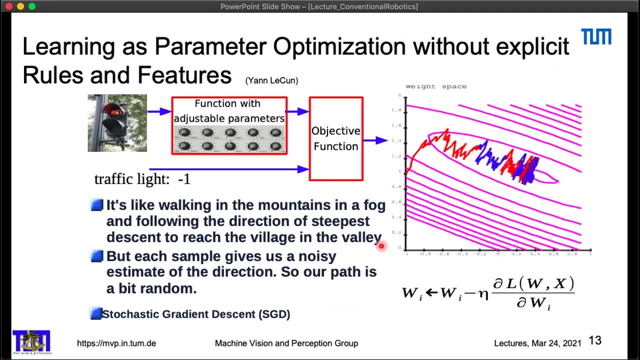 the one from him and that you have multiple layers which can be trained to. for example, do here labeling of this picture to decide what's in the image and you what's the first thing, which actually is very dangerous, and the whole thing is that you don't really try to understand how the learning is is done for now, basically most. 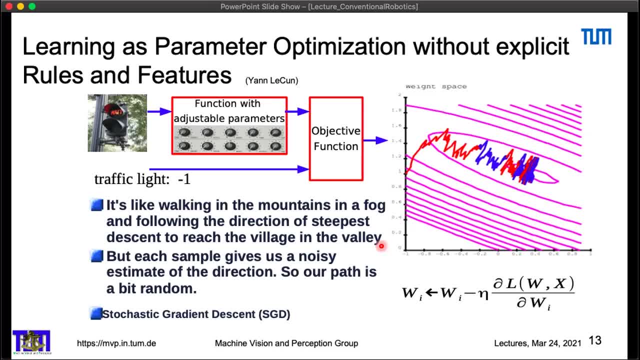 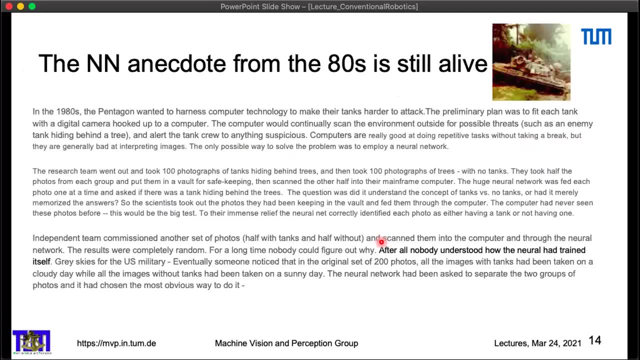 people are just training until the loss function basically meets some criteria and then the system is kind of okay for them to use. so there is no, no real science okay beyond this back propagation here, how to do it. and you know, i was very surprised when i was, when i was doing my phd- 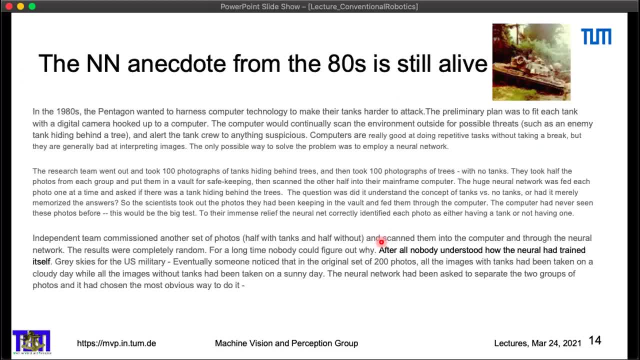 there was an anecdote. i will give you the text later, so it's just for so, basically what? what this anecdote was saying is that you want, they wanted- to build a network discriminating between friendly and enemy tanks in images. they took 1000 images. they took, they split them into parts. 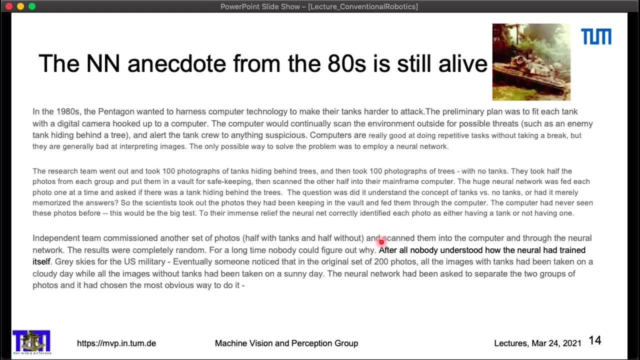 500 for training, 500 for validation trained the network. back then training was really difficult because there were only binary networks. in the end the network was trained on the 500 to distinct, discriminate between the two types of tanks, applied it on the other 500. work beautifully returned to the funding agency. they tried again and this thing was not working. 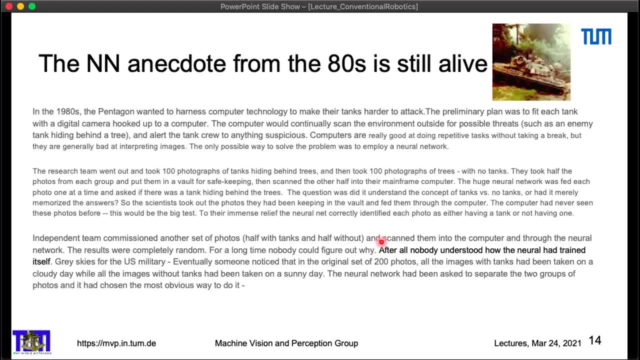 so took them quite a while to figure out that the images they took for the friendly tanks were taken on a sunny day and the images taken for the uh enemy tanks were taken on a cloudy day. so what the system trade? what the system actually learned is to look for clouds. so it was not really tank detector, it was cloud detector what they built. 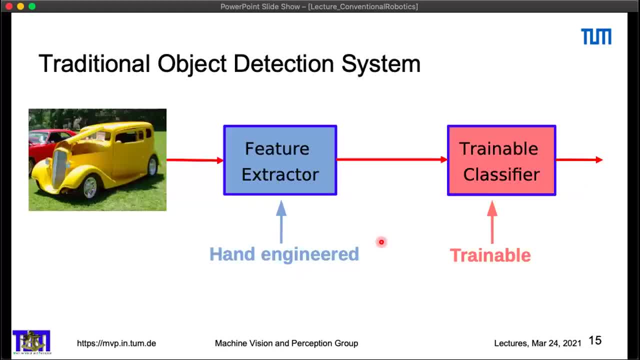 without even knowing you would think does not happen today. well, let's just have a look what can happen in such a system. so here is a traditional object detection system. you have some feature: extract extractor, sift, surf, brisk, whatever maybe you. so these are the features. when i was 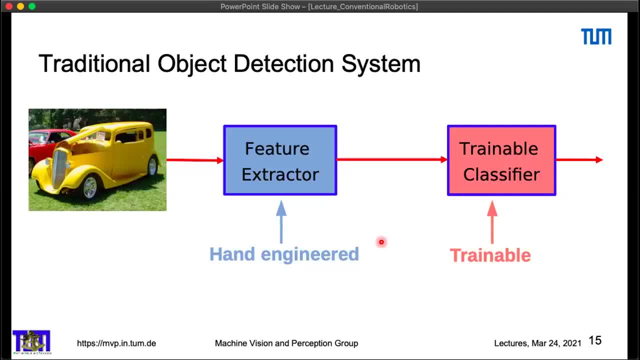 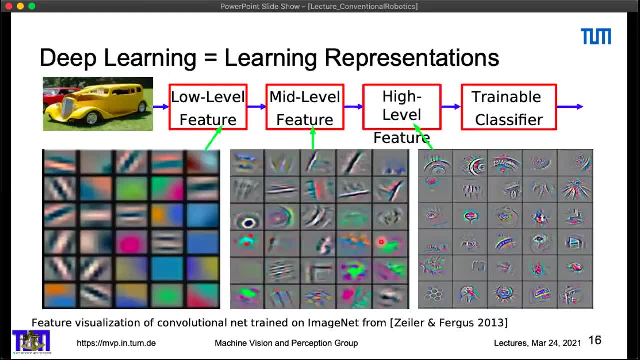 young and the dinosaurs ruled the world. we were using them for object recognition and then you have some classifier which just merges them together to say, oh, that's a car. people say, well, you know, i understand what my network is doing, because if i train a set of 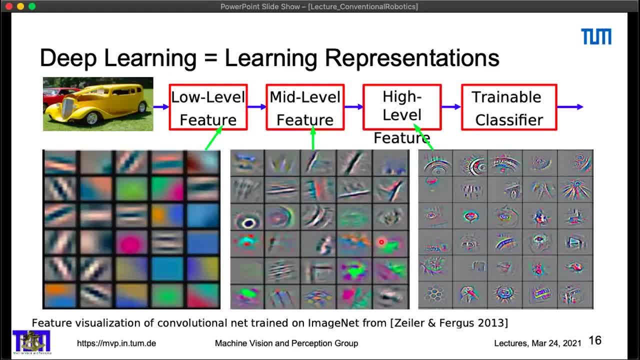 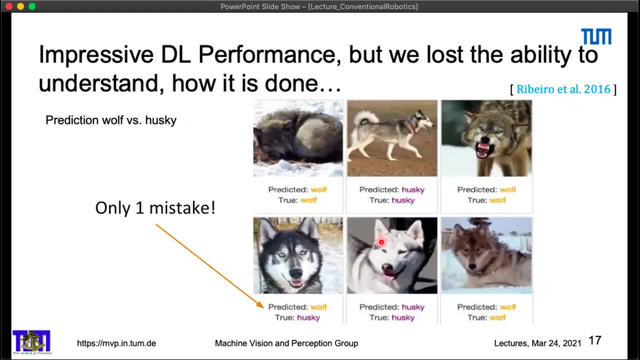 fully connected layers or connected layers. i can see that the first one is a low level feature detector, the second one is mid-level, high level, and then there is a classifier in the end. so actually they feel like they understand what the network is doing. but, um, this gives us really pretty nice performance in the system because, well, you know, this is. 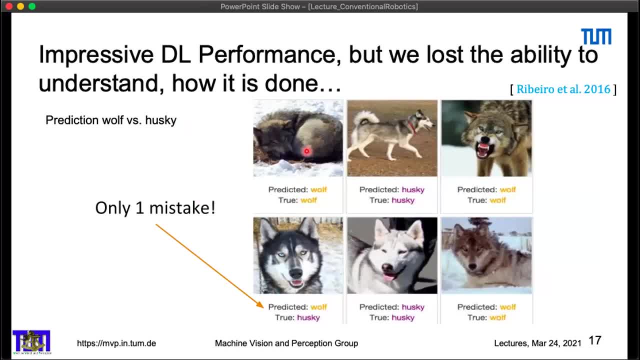 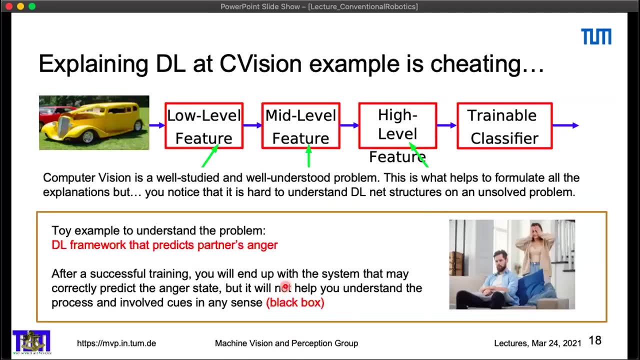 an example. you may know it already that this is a classifier which is supposed to distinguish between wolf and husky, and the system works beautifully, beautifully here, makes just one mistake: misclassifying here the wolf for the husky and using these explanations, basically, people feel like they know what's going on. the problem is, vision is something which was 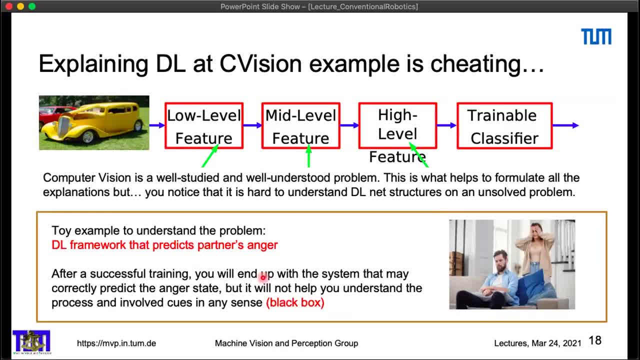 well studied before the deep nets started. that's why they can explain what's happening, because we know basically how it's done. i've actually challenged people to try something different, to train a network to predict the partner's anger. just find cues physically what's happening to. 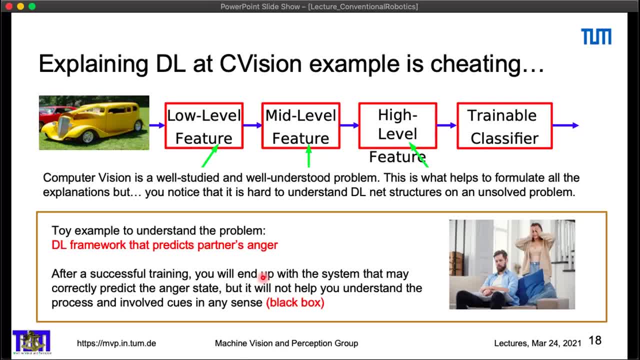 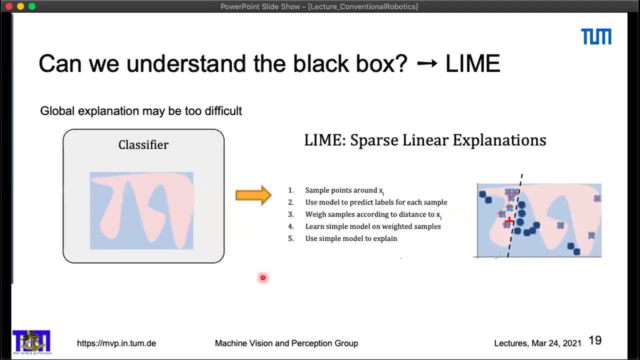 decide if angry or not, and after successful training, the system was doing the right thing, but you still could not explain what cues it's using, just because you didn't know it before, and the performance of the network was not really helping. so what people should do is actually try to understand what's happening in the network. 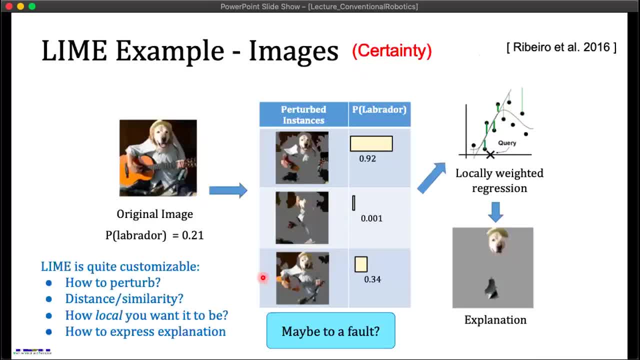 it's very tedious because it's a very high dimensional system and there are ways how to actually find in a find which cues the system is using to make a decision, just by perturbating the image appearance. here an example of the dog with the guitar and you see basically which. 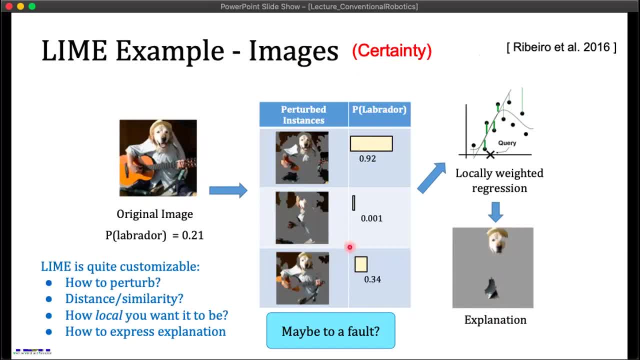 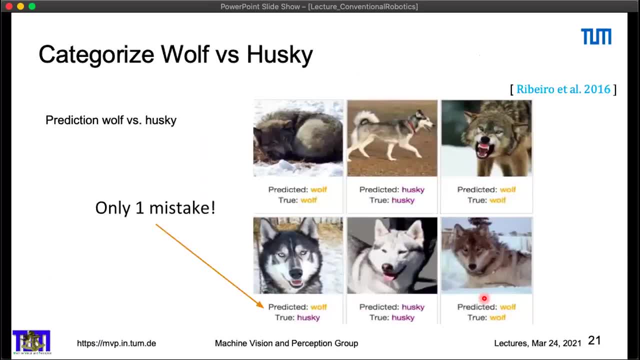 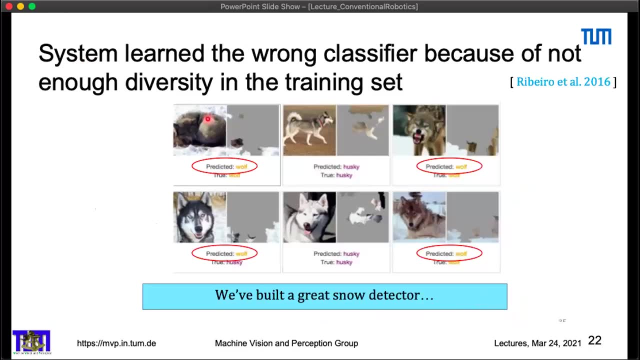 parts of the image actually were used to decide it's a dog from this image. the network was using just the head and part of the body here. now going back to this wolf versus husky: here is exactly the same thing: the image and which parts of the image were used for classifications. 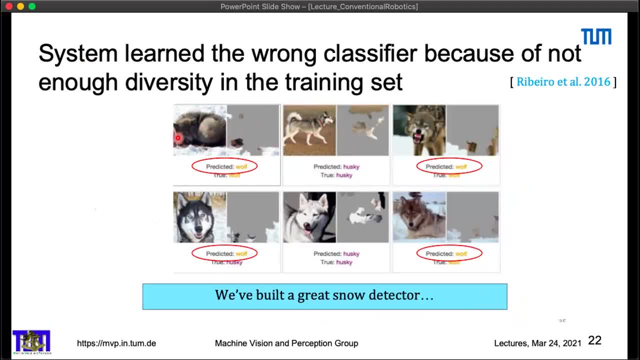 and when you see here for all the wolf examples, the system was not really looking at the wolf, it was looking at the snow. by accident, all the images was had snow in them. so the system was really just saying wolf each time there was snow in the image. so you see the right image here. it's always what, this, what? 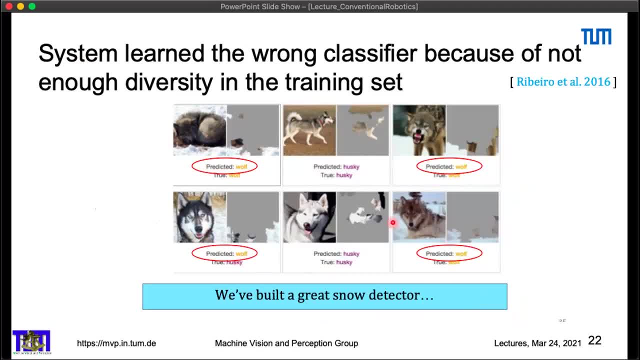 the system was looking at. and for the husky, the system was actually looking- no, sorry, the other way. for for the wolf, the system was looking at parts of the animals. so here, here and here for the. for for the husky, the system was looking for the snow and the misclassification happened, just basically. 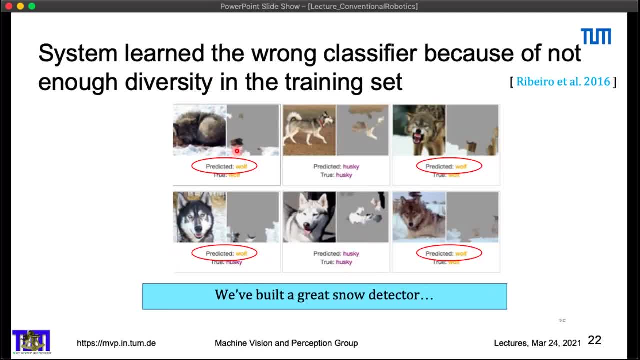 just because the wrong cues was learned by the system. so you, if you don't validate what the system learned, then you may build something which may not behave correctly in your application. and if you want to make decisions on the robot, you better know what's going on. and you can't do that. 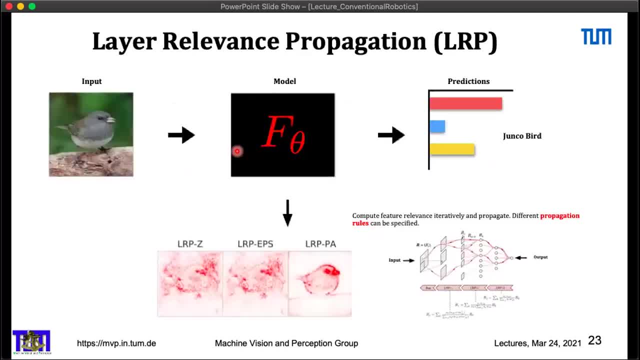 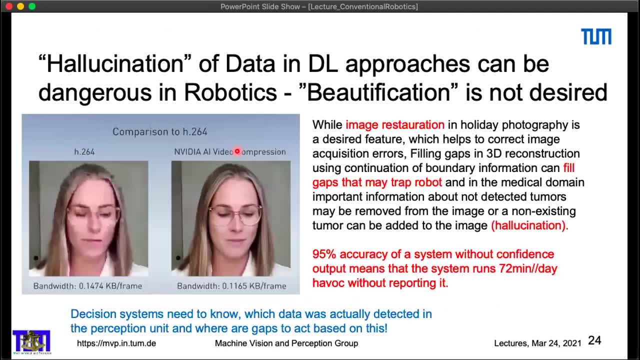 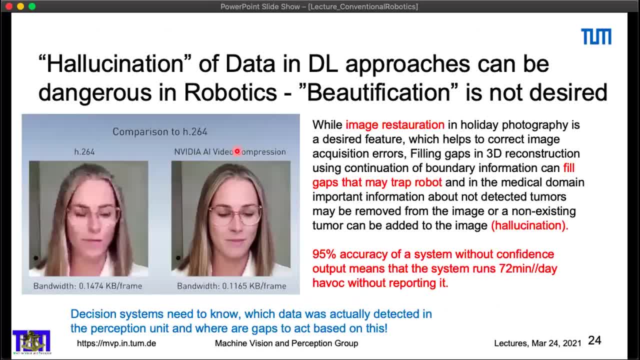 example, deep learning for medical domains to do image restorations, and the danger is that in the, in the areas where the image is distorted, the network is providing your information from kind of an average appearance in the region. so just imagine there is someone with a cancer area in the body and this part was not correctly sensed by magnet resonance or 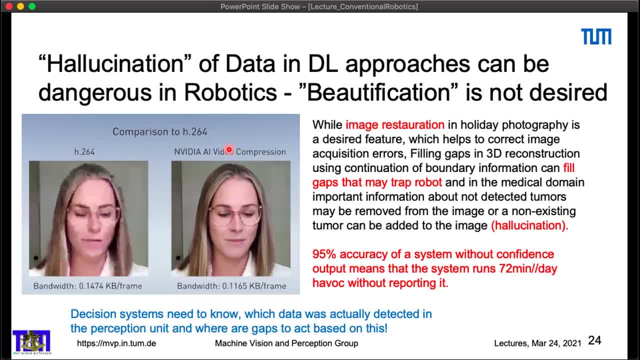 whatever. now, your deep learning system made a beautiful picture for the doctor from this just by in painting an average appearance from this region without looking what the patient is. this thing's very nice for the doctor but it's very used. it's pretty much useless for diagnosis because 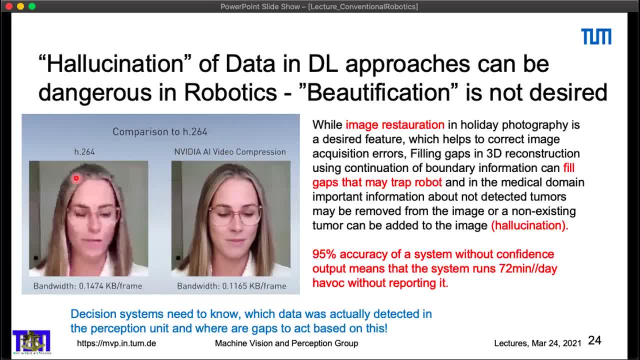 you miss information. another funny thing, which i think is very important, is that the doctor is not the doctor in the dark enough, and so the doctor is not as open about the patient as he is now. so there's a problem with this method in which i noticed, like recently, was this nvidia compression? 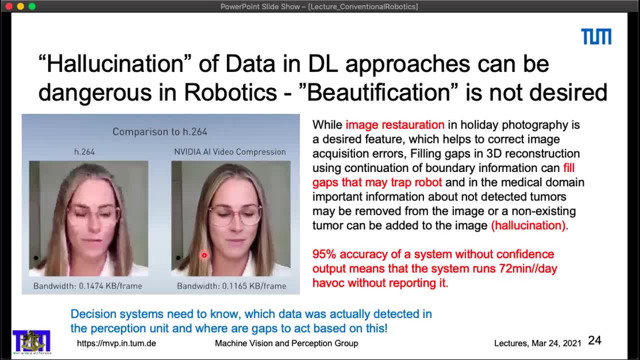 where they were trying to in to improve distortions in the image. so this is the distorted image, this is the improved image. it would be nice to see if you find the problem with the system here. if you look at the nose of the woman, you will see that she got a plastic surgery between. 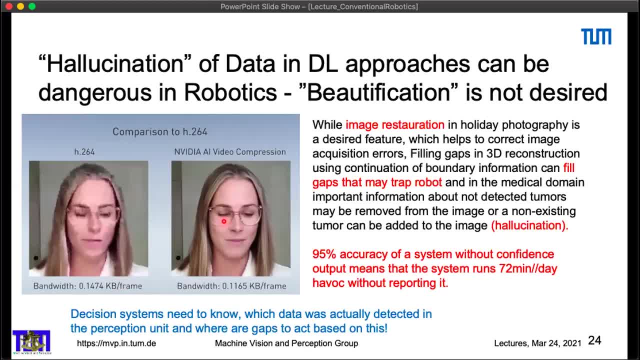 And then the system does? they used, of course, people with different facial properties. Her face looks completely different. It looks nice, but it's not hers anymore. So this is what happens in environments, And now basically applying it to robotics. 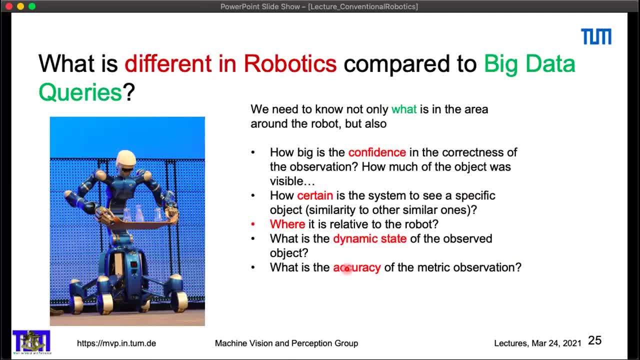 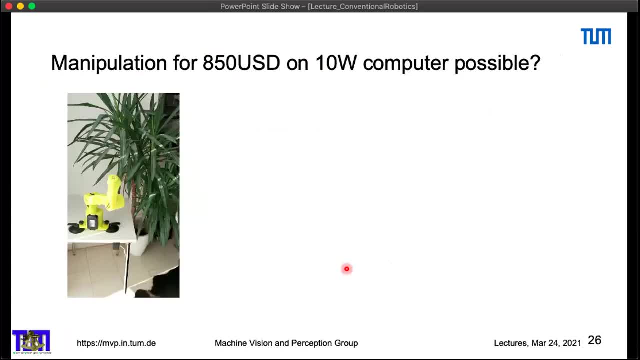 This is adjusted robot from DLR, which I work with, So it's a humanoid robot with 46 degrees of freedom And we would like to apply it now. This is something I actually just built. You may see the robot still behind me. 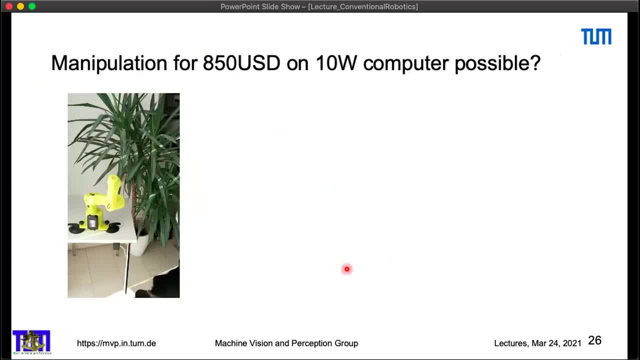 this yellow thing It's. basically people always think that they need very expensive graphics cards to run systems on the robots, So what my challenge was is to build in three days a manipulator which can see and manipulate. So the first thing to do is basically get the robot. 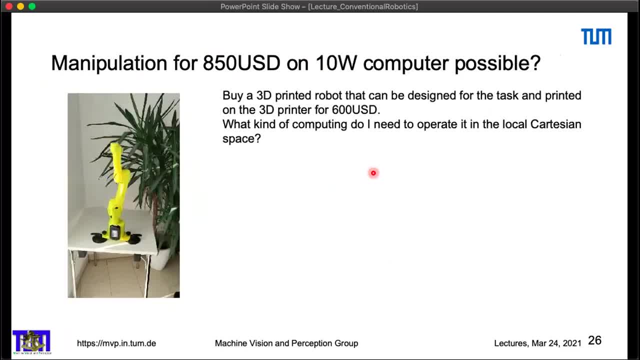 So I got the robot- a 3D printed robot- from friend of mine who has a company here in Munich for $600. So this is something which can basically control by now. the question is: what kind of computing do you need to run such a robot in the environment? 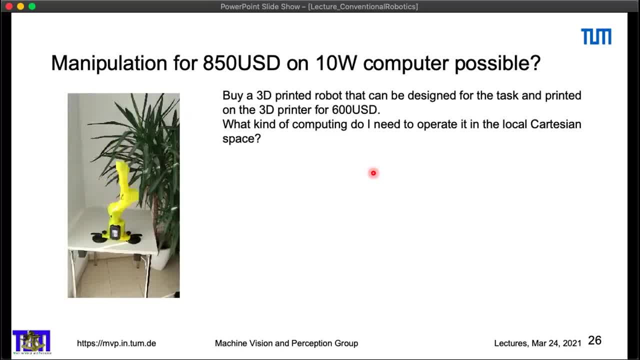 So do I really need my graphics card to train it to use a million examples to actually understand how the robot is moving? No, I don't. All I need is a small Raspberry Pi computer which talks to the robot And the whole thing which you would train. 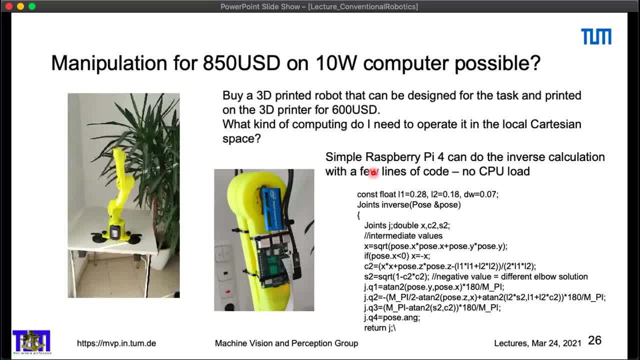 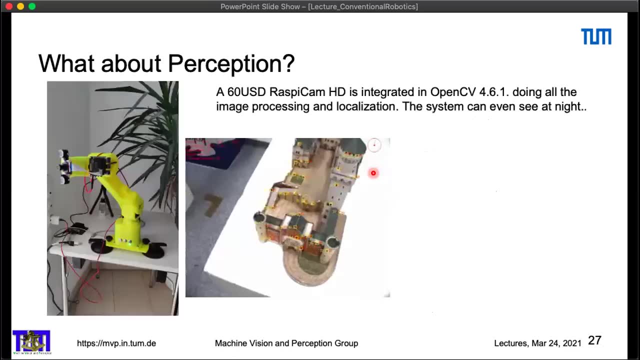 is actually something which is known to man. how to do it. These 10 lines of code actually is everything you need To combine position to joint space and run the robot the way you see it in the image. So of course, the robot needs also some input. 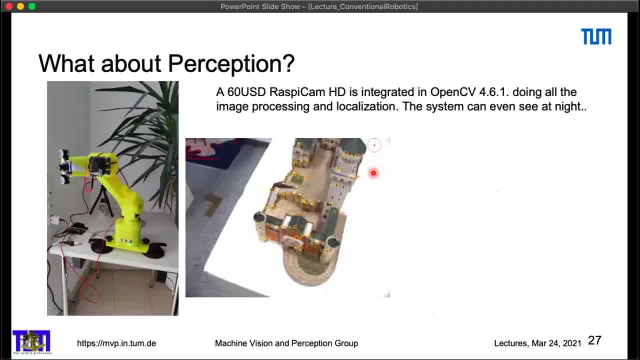 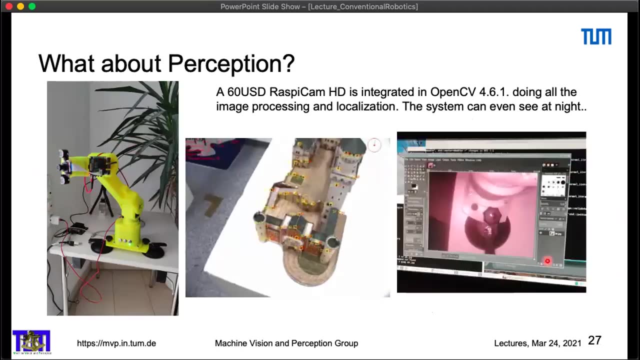 So do I really need the graphics card for the perception part? Well, what you see here is basically a Raspberry Pi HD camera mounted to the Raspberry Pi computer controlling the robot. This gets you directly To the image, day and night, And it can be used directly to calculate. 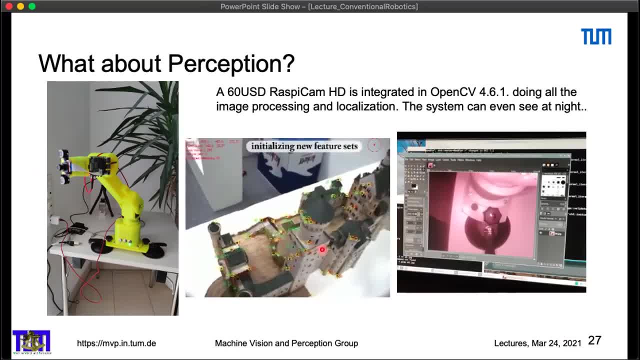 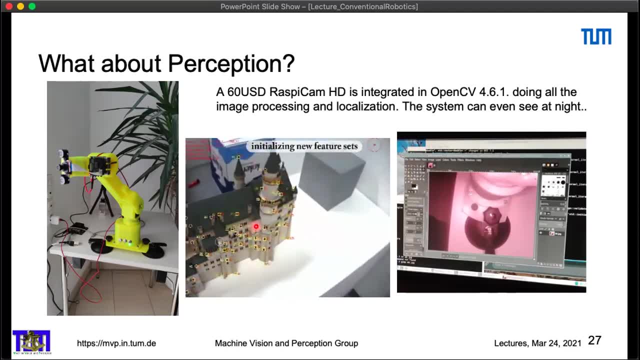 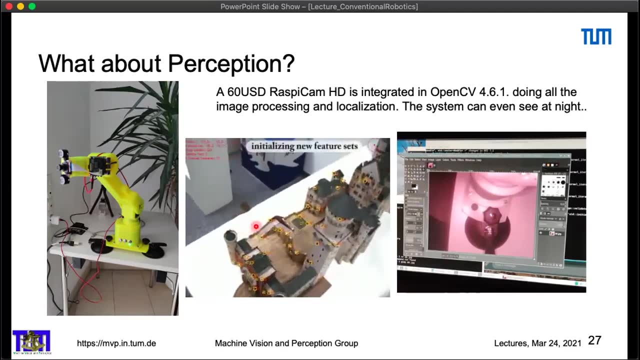 the pose of the robot, So I hope you can still see the small yellow points. Basically these are track points of the robot And the system gets highly accurate 3D information about the pose. Everything is running on the Raspberry Pi here. 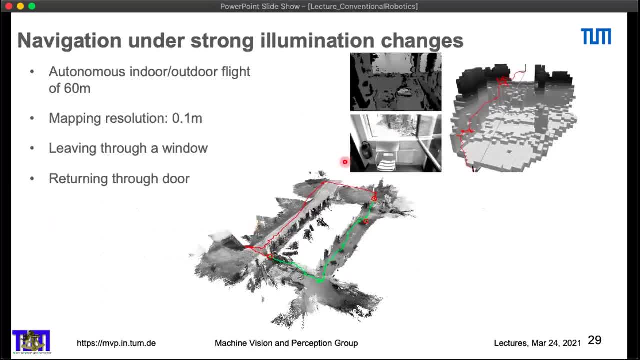 And just to show you that it can be used also in other settings. Let's see. This is a system which we used 2012 on the drone. Basically, the system was starting here in a container. This was a lab container, Was basically looking for a window. 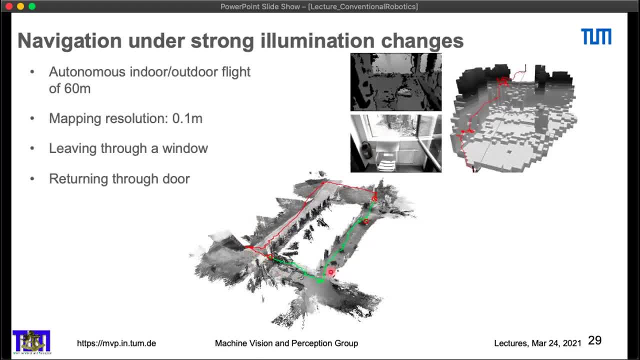 flying outside of the window, flying around into the house and flying back to the place where it started: 2012.. All navigating from the perception. So basically everything was running on a small. back then it was an armed five big board. 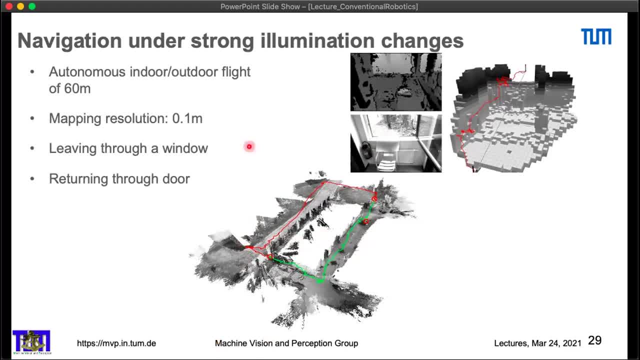 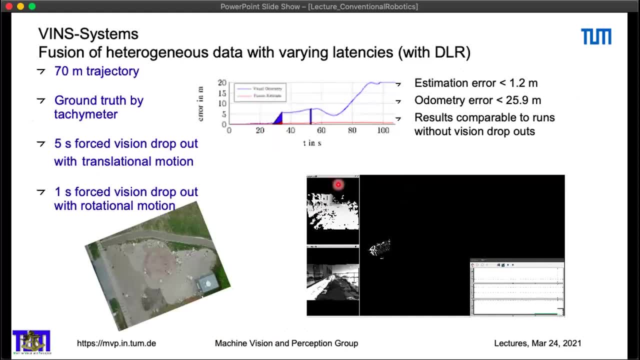 And the system was able to do this operation And just because you could restrict it to something which was predictable. Same thing here is basically: if you do perception, you should not be using perception just by itself for control. You should fuse it with your own expectation. 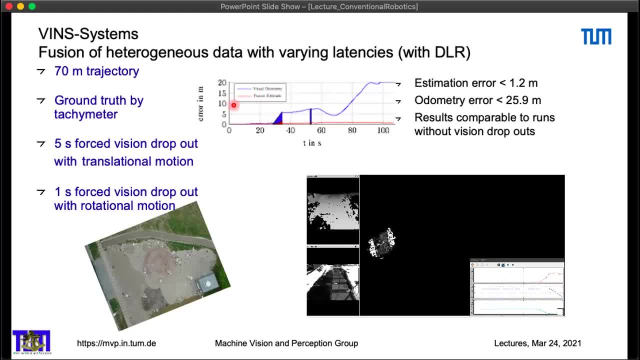 just to make it more robust. And you can fuse information Only if your perception gives you not only the value itself, but also the covariance and accuracy of what is happening, And this helps you to deal also with situations where the system may be blinded, for example. 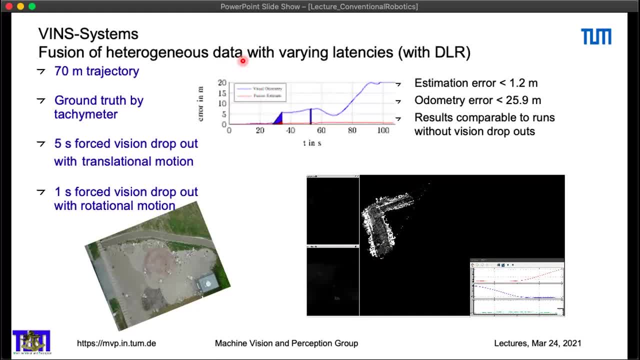 or maybe a failure in the system. So this was the system flying basically on a 70 meters route with really severe sense of failures. We switched it for five seconds during translational motions and one second during rotations on a flying drone, Because this is a lot of work. 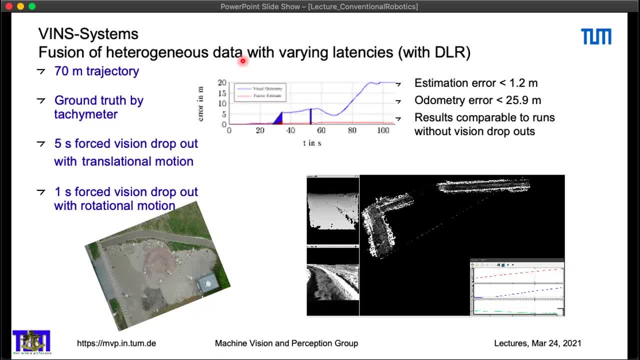 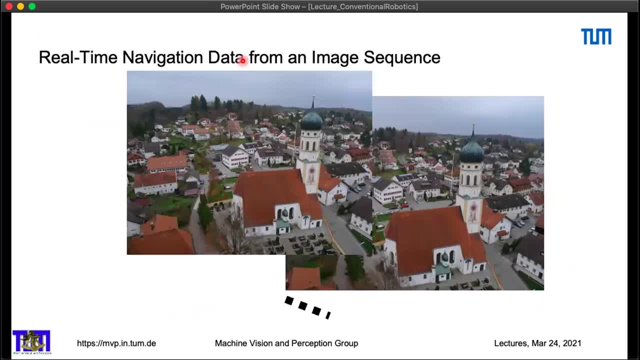 This is a lot of time basically to lose your position And the system was able to recover. We use it also now to do reconstructions, And you see a lot of people now these days learning how to do reconstruction. Well, we've done it in 2007 from a drone. 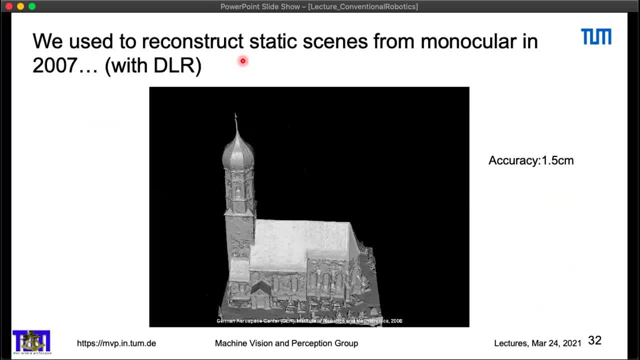 We took 60 images from the drone And, using structure from motion approaches, basically stitched them together to something which is accurate to 1.5 centimeters. So if you look closer, you see all the thumbs. the thumbs you see even the solar clock on the church is 1.5 centimeter. 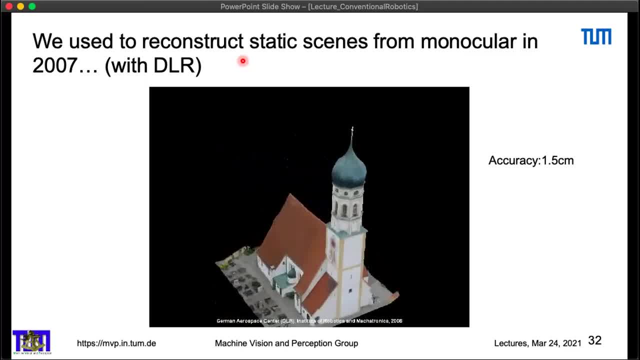 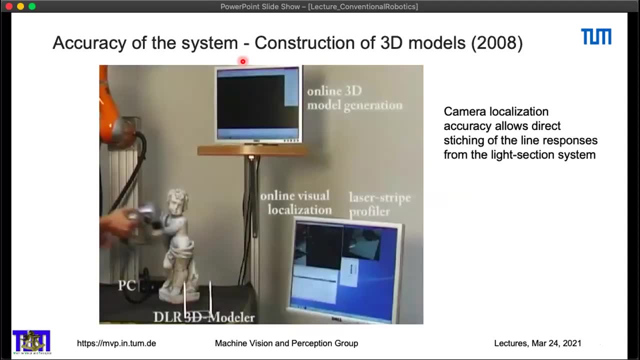 accuracy And no training required. You just take the images, you stitch them together, you calculate the 3D And it works in all environments. To do the accuracy. we really built a system now which can also localize based on such feature observations. 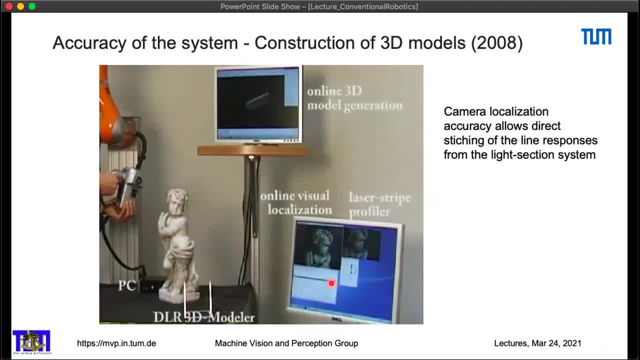 So here, what the system is doing is projecting basically a laser line on the statue, So you have, in each image you reconstruct, one 3D line And moving the sensor down, you stitch the lines together And the localization of the sensor. 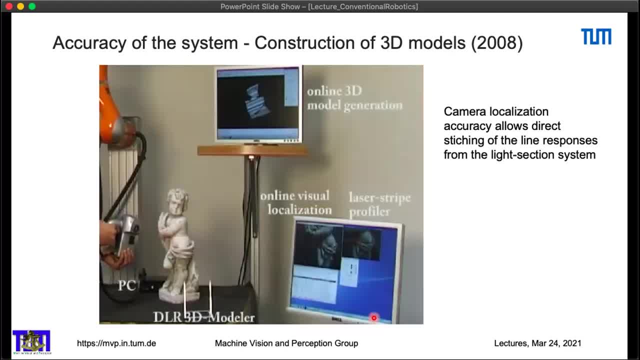 was accurate enough actually to stitch them just without doing any post-processing. So the 3D structure you see here are single 3D lines stitched together, And to do this robustly, you just fuse this with an IMU, IMU. 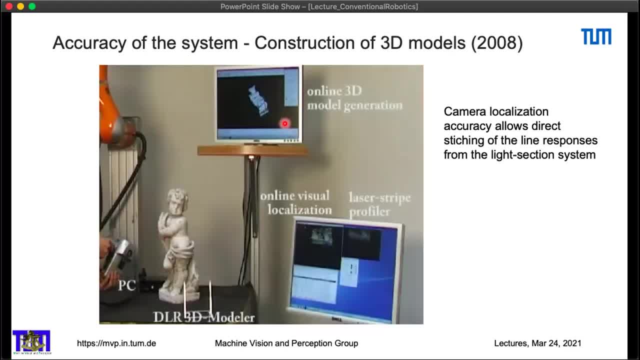 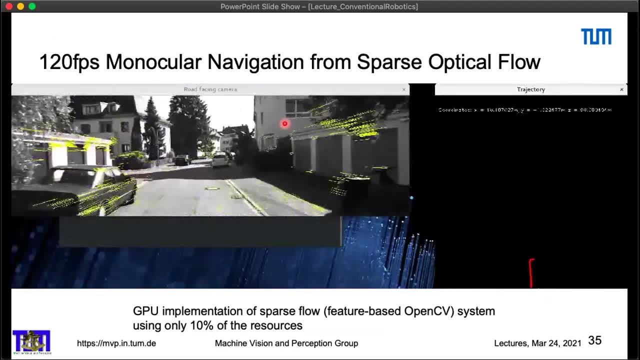 IMU Sensor fusion is something very important, And you can fuse the sensors only if you really know more than just the value itself Here. this is something which I'm always like if I look at what power you use in your current systems. 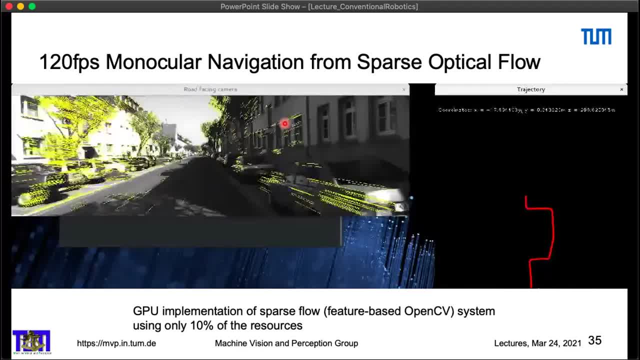 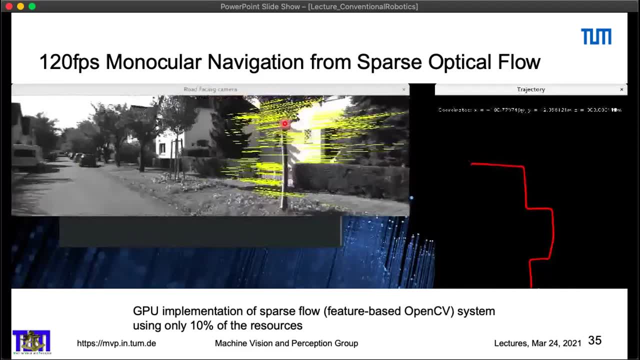 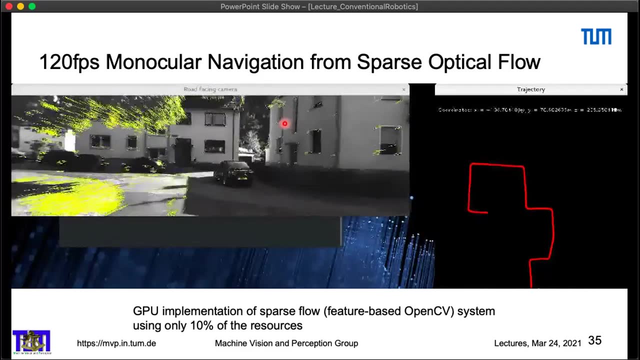 I'm always amazed. So, like for fun, I applied my navigation system I used on the drone on a graphics card And this is running 120 hertz localization using just 10% of this Of the graphic performance. So this was TI 2080.. 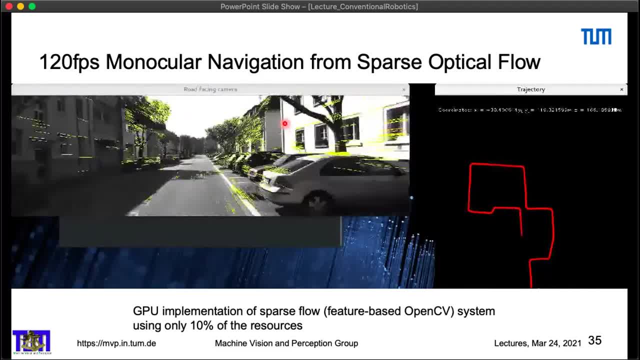 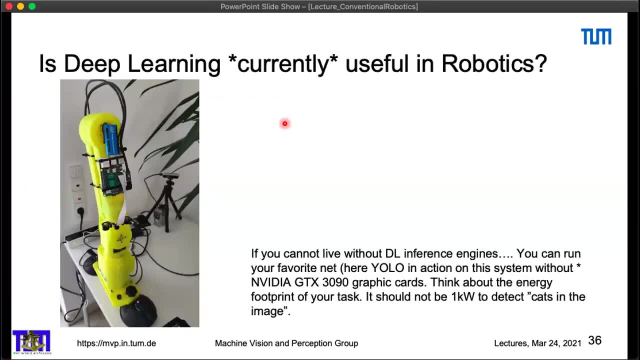 And I used just 10% of the GPU to run the system, giving me the position and also the orientation. But back to the robot So we can localize. The question is: is deep learning completely useless for robotics for now? No, it's not. 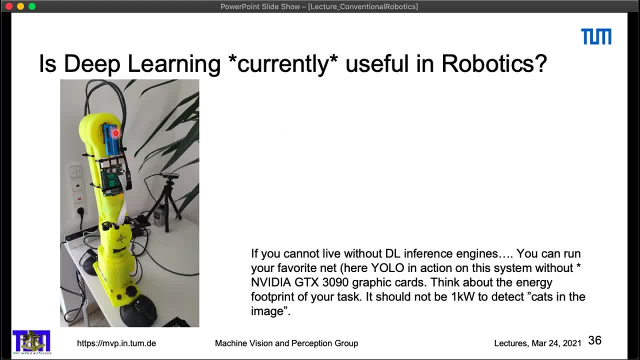 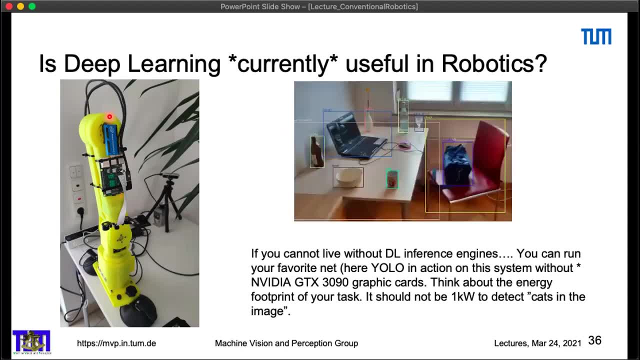 On this system. actually, I have here a small neural stick from Intel where I can move the interference from deep learning And I use it to draw attention. So this is what deep learning is perfectly fine for: To focus processing on some sub regions in the image. 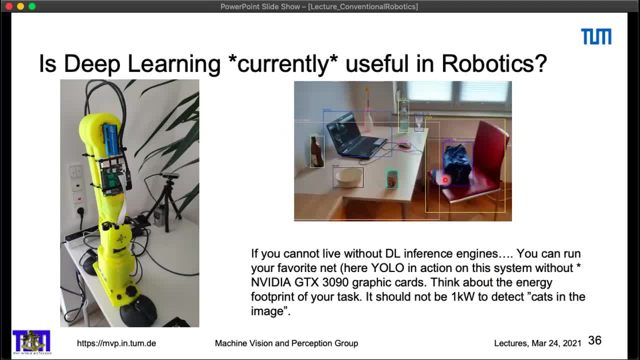 So the system is telling you: here's a laptop, Here is a bag, Here is a cup. And now, depending what I'm trying to do, I really can focus now the other processing, To focus now the other processing To do it with 3D information and to interact with this. 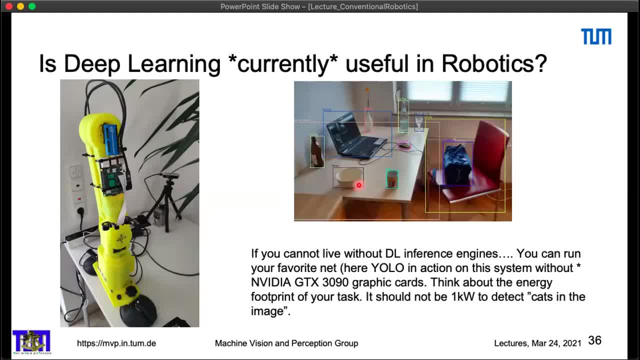 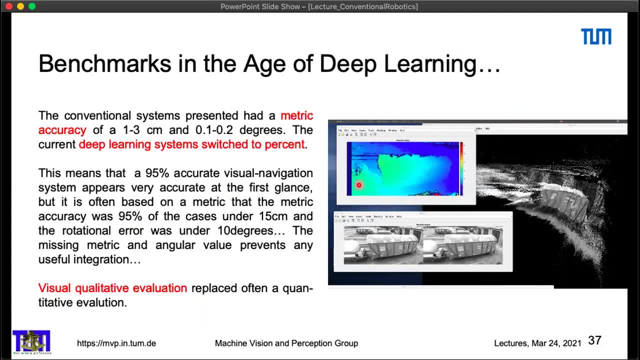 Just because the interaction from now, from deep learning, is still not good enough. to run the manipulator, The benchmarks, is also a big problem in learning. So what I'm always amazed is that people are usually showing in papers the real image and the depth image. 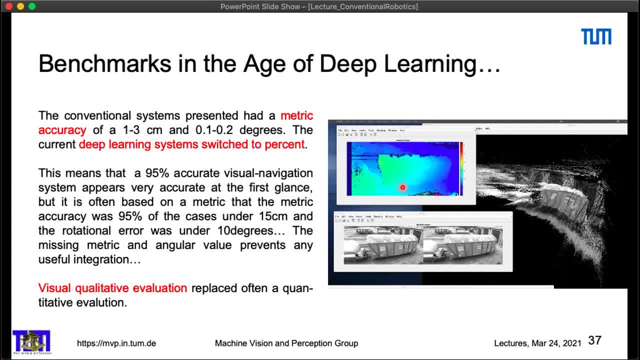 And they claim now that the system is working. So if you compare these two- this is a car from a train And this is a 3D reconstruction of the car- You cannot really tell the error in the depth image. You can tell the error only if you. 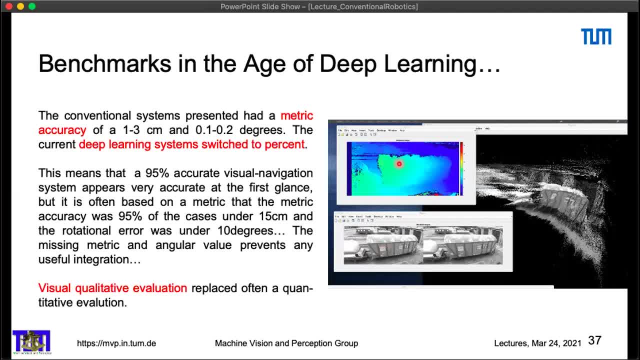 reproject the grayscale onto this depth image and create a 3D point cloud out of it, And then you see how good or how bad it is Here. this was actually not deep learning, But this was coming from a stereo system. I had a tiny rotational error between the two cameras. 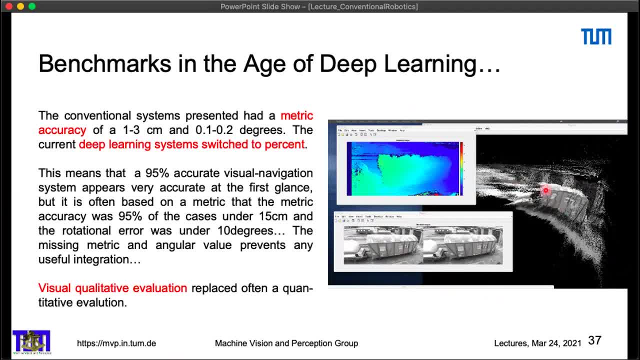 And this resulted already in a very large distortion of the result. I don't see anyone looking at any orientation errors these days. People are always just providing this. So really, the benchmarking needs to be improved to actually really understand what's coming out of it. 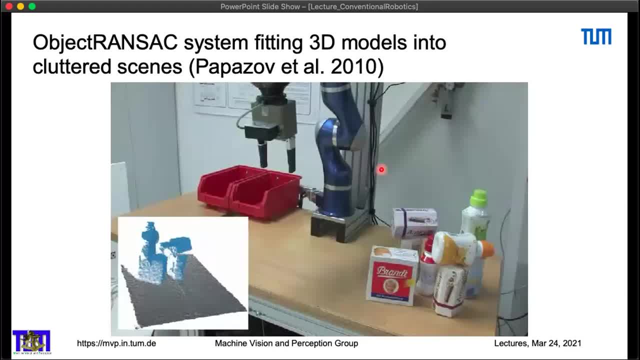 Just to show you what's actually possible, this is 2010.. This is basically a robot which gets 3D point cloud from Kinect- back then This was the old real sense- And it's matching into this point cloud objects. It's behaving. 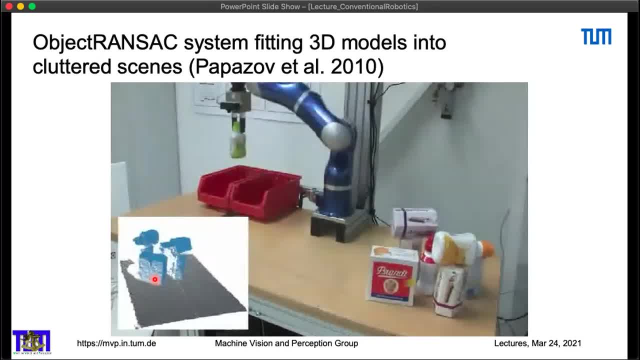 It's a database of objects and can deal with cluttered scenes. match the objects, gets the position and gets also the function. And now the system can be used to sort objects in the scene. So it's basically putting the chocolate boxes in one box. 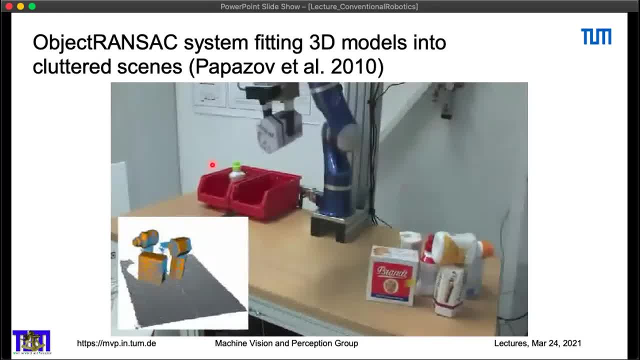 It's putting all the bottles in the other box and so on. The nice thing about this is I know for each object how much of the object I've seen. This is really a cluster, a clutter, And some of the objects are visible only by a small part. 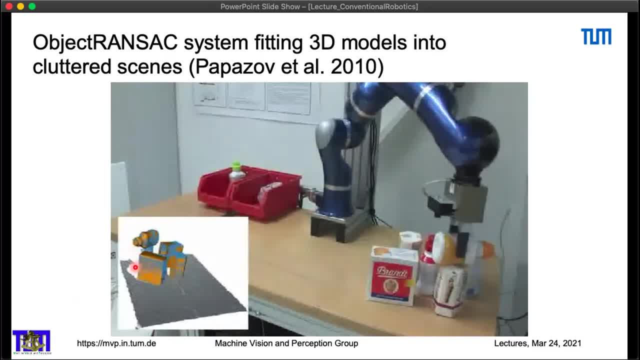 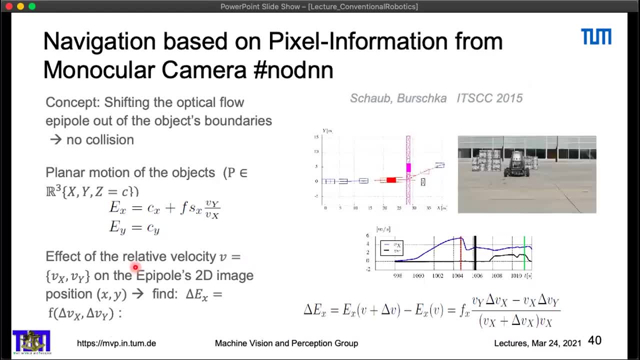 So I can always decide: do I really trust the system or not? And I get also the 3D information. So now a little bit more modern project. This is something which is, I think, a very nice way of applying biological vision to systems. 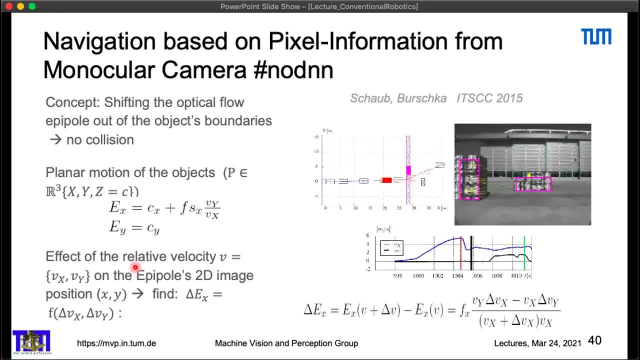 If you skip completely the metric information in your system, you can suddenly drive a car with a monocular camera because you don't need 3D. What you need is the information when you will collide with the system, And the collision time can be directly derived. 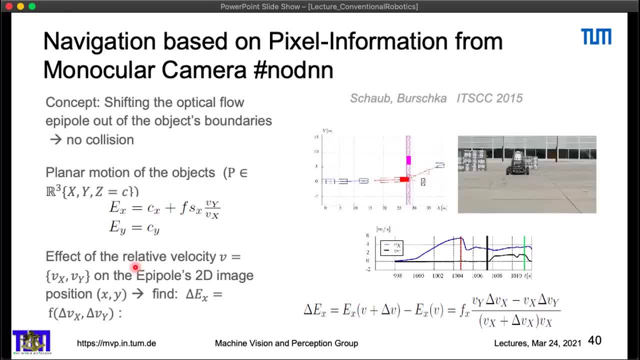 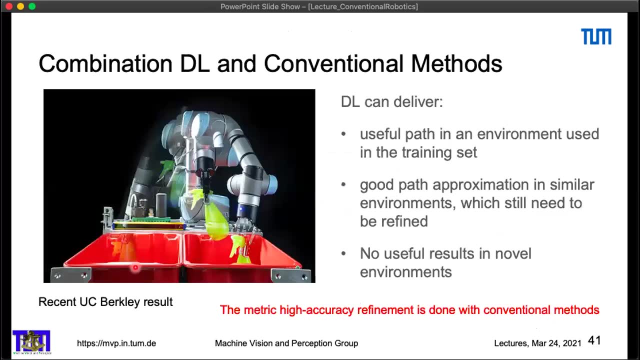 from the pixel information in the image. So we are driving this fancy car you see here completely from a monocular camera, uncalibrated, So you don't even need to calibrate the camera. The system really can avoid static and dynamic obstacles. 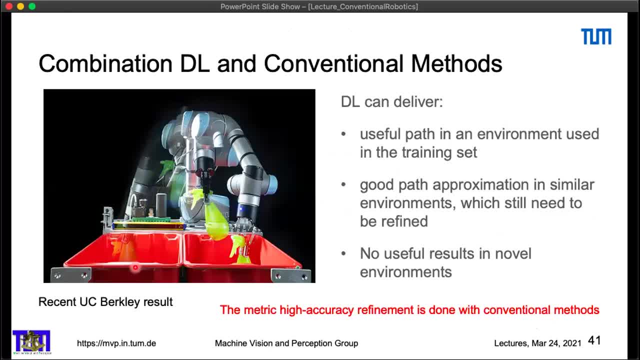 But, as we've seen before, it makes often sense actually to combine these two. A simple example was what I was trying to show with this object recognition. You use the deep learning to actually draw attention to regions in the image, And then you use conventional methods to refine it. 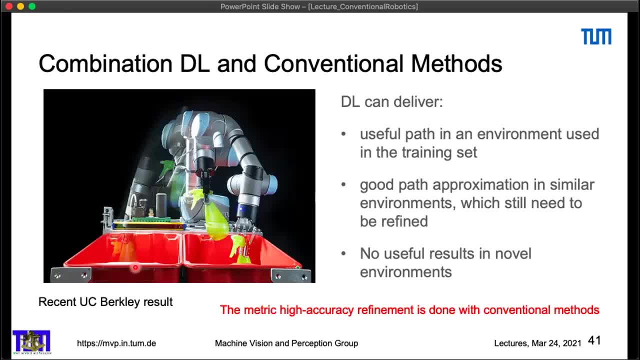 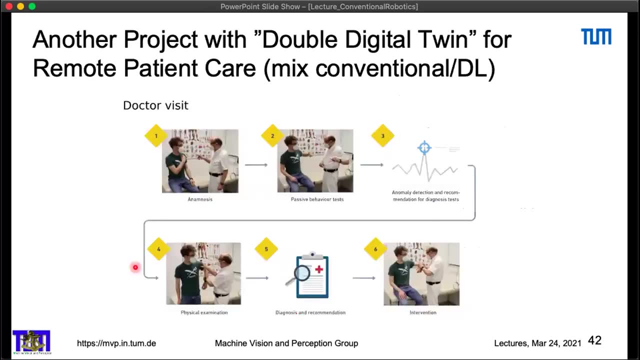 It's not only me doing it. Here is a recent Berkeley result where the manipulation from deep learning just didn't even work. It was always having some remaining collisions, But it was giving a good starting point, avoiding a lot of processing in the conventional method later. 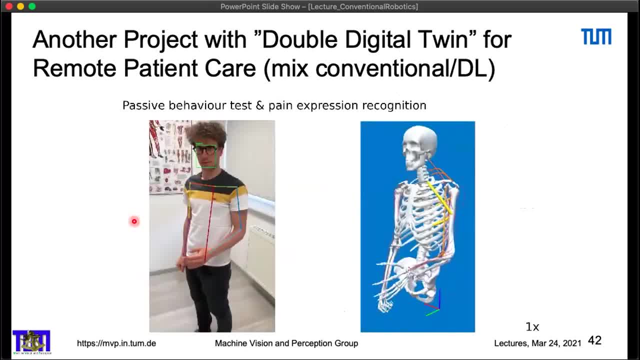 And this is something we use also in our system. This is a system to two robots. One is in Garmisch-Partenkirchen, 150 kilometers from Munich. The other robot is in Munich, And the goal is basically that the doctor in Munich 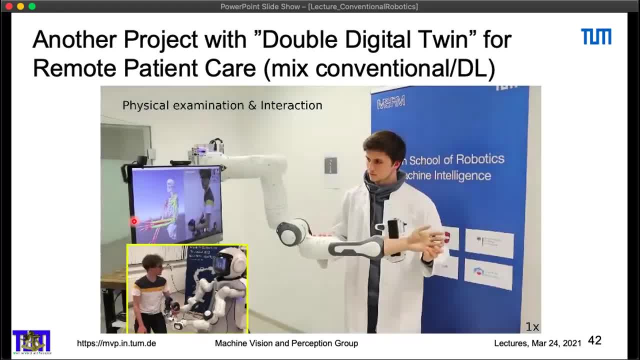 is inspecting a patient in Garmisch. So the two robots mirror the forces and the appearances of the doctor or the patient on the box on the site. You use here deep learning actually to get, for example, a skeleton of the patient. 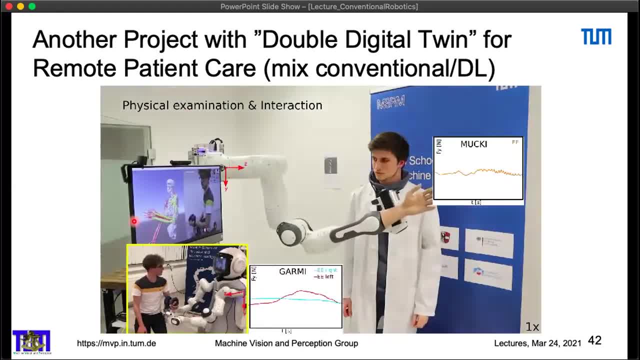 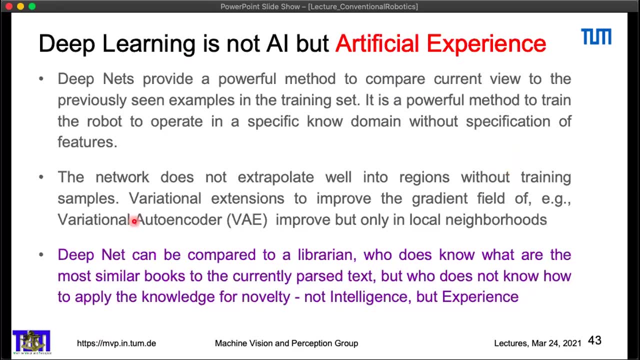 It's a lot easier to use open pose to get skeleton than try to do it in a conventional way. But all the control and all the decisions are basically done based on conventional methods, just because we need quality values for the robot And just to keep on time: one minute. 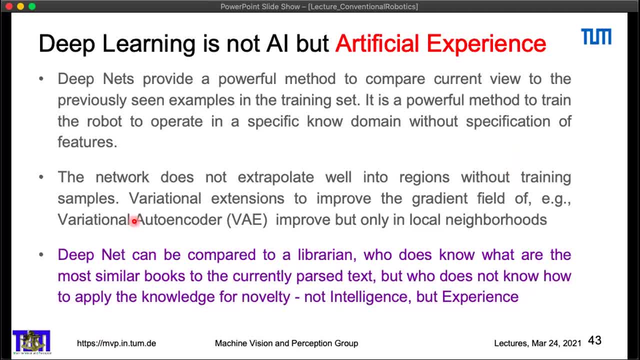 So for me it's like: OK. So basically, deep learning for me is still not AI, but a different experience. I'm happy to discuss it. So basically, they provide a powerful method to compare what you currently see with a large amount of data. 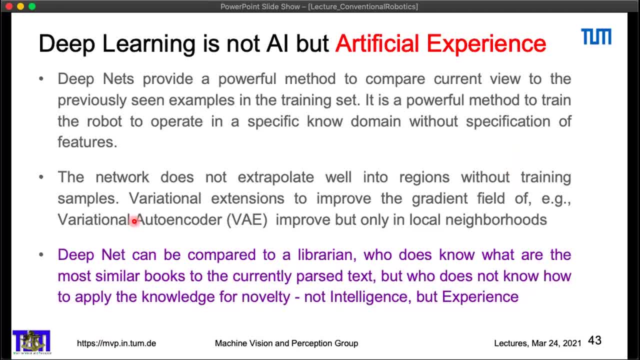 No wonder They were developed by companies who had to deal with big data. That's what they are made for. The problem they have is, of course, they cannot really well extrapolate into regions they haven't seen before. The conventional methods are doing pretty fine because they. 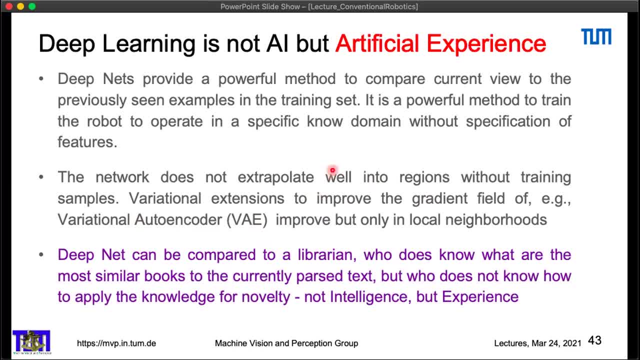 have a lot of data, but they don't have a lot of data, And so they're not going to be able to do that, And so they're not going to be able to do that. So there are rules, you build. The difficulty is just to build the rules first. 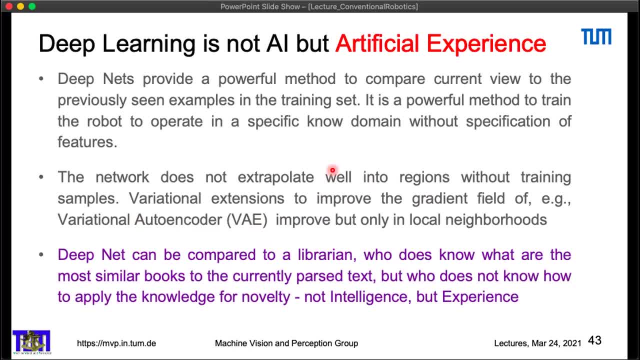 And what I want to say. the deep net is: for me it's like a librarian. It's telling you what you currently, what's a similarity to what you see, to what it has seen before, But it still didn't learn anything. 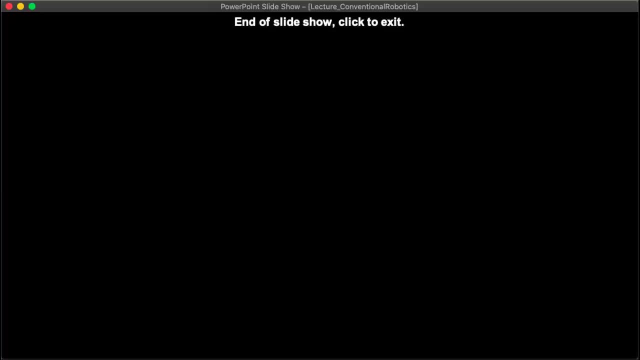 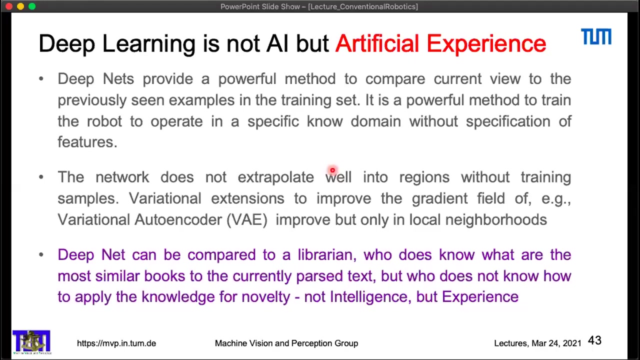 So it cannot really derive a new approach from this. So half an hour. I'm pretty sure that I will be eaten alive now, but I'm fine, Thank you. Thank you so much. Lots of different projects, lots of different things. 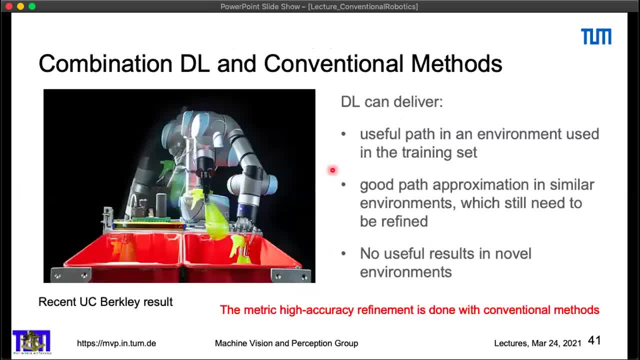 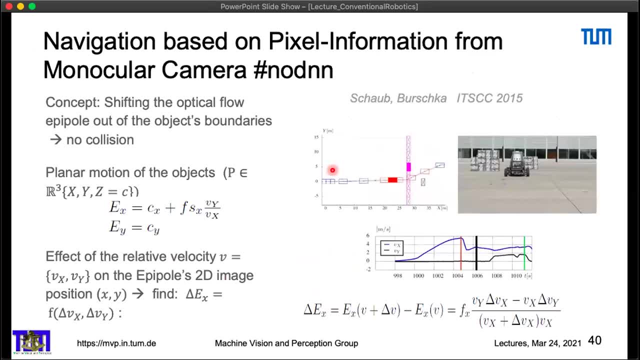 Well, I skipped a lot of them. I still have more So, but I wanted to actually kind of focus on perception for control, So maybe it was not so visible in the talk. I have a question there. I mean I'm sure the students have to. 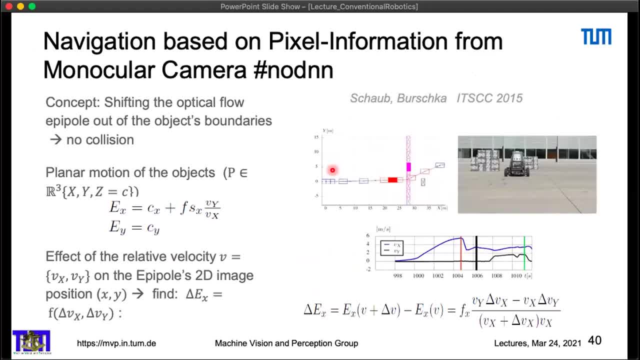 Maybe I shouldn't go first. Well, maybe, while they're thinking about other things, to ask: how do you choose your project, Like, what ideas do you work on? Or what do you want to apply robotics to next, or something like that. 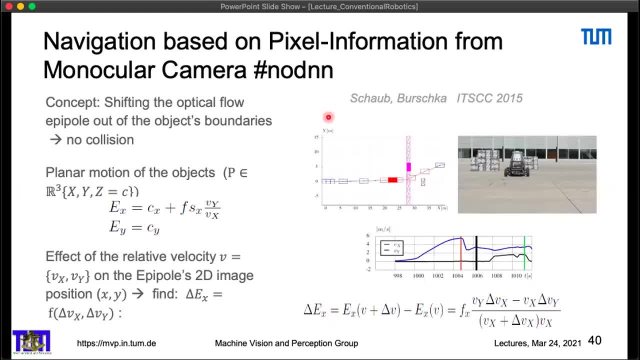 What actually, as you've seen, back in 2007,, 2008,, we were working on geometry, how to recover geometry, How to have the structure, Because to operate a robot you need to know where not to collide with. 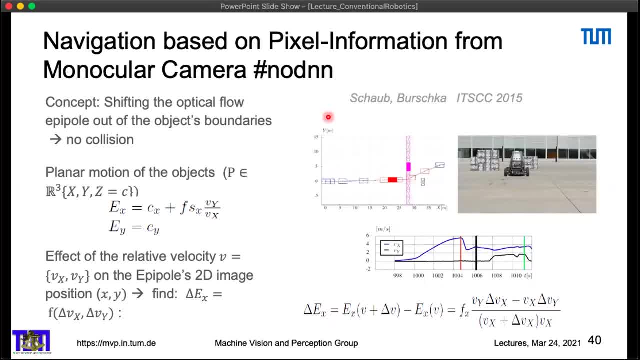 But for most things you don't need to know what it is, You just need to know there is something. So once you start doing something in the environment, you need to know the semantics. You need to know also where are things to label them. 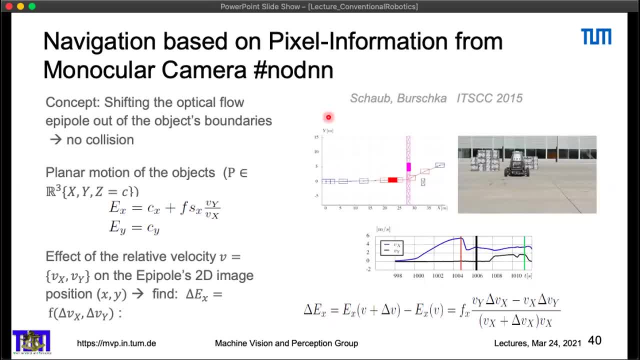 And this is what people also have been learning to do, But I think this is sorry to say, solve problem. So the challenge for me now is really understanding dynamic actions and plan in dynamic environments, And this is what I'm doing a lot now. 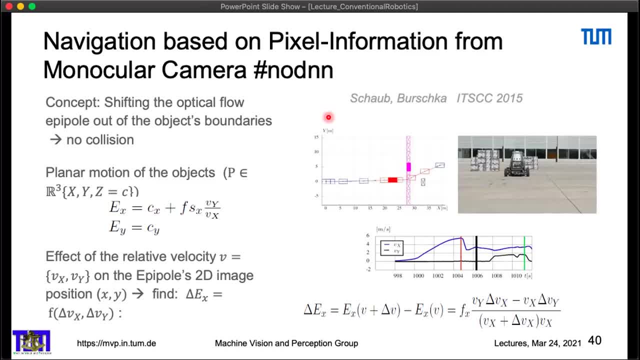 So I have really two PhD students working on car projects, how to actually interact with pedestrians, how to do safe planning in a dynamic environment. And you will be surprised, the system can really predict in a very robust way the collision areas, Although the trajectories are very different. 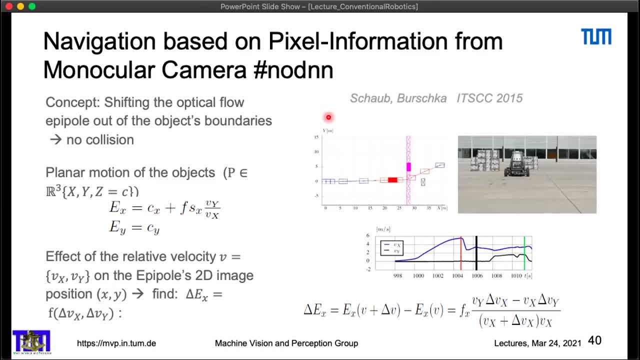 I'm actually. the system I developed for cars will be applied now on the novel plane we developed with some other company And this is a sense and avoid system. The pilot has really a big challenge to understand if he or she is colliding with someone. 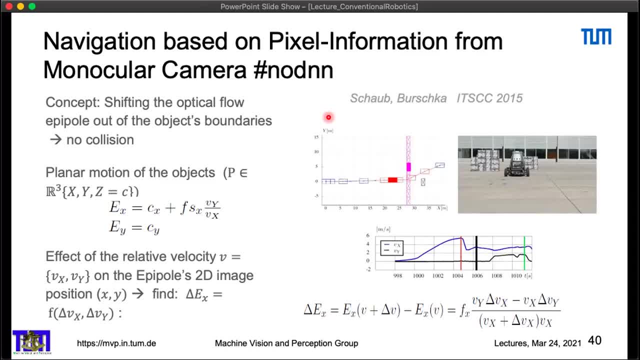 flying around And the system is really drawn to draw attention to what's happening. So the kind of thing is basically planning in dynamic environments, understanding actions, understand the action context. I have a German heart center project- I've skipped completely here- where 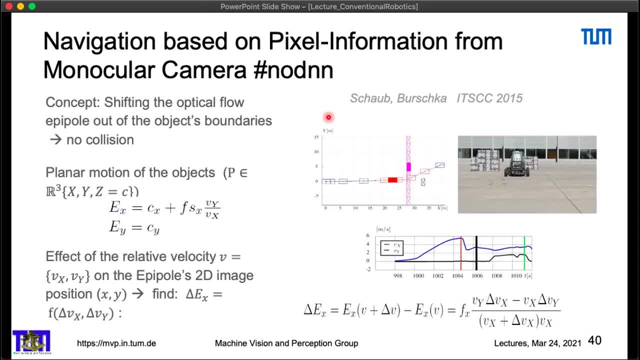 I'm actually writing an automatic protocol of what the nurse or what the doctor is doing. just to save them, They have to write down everything they did, And this is a very tedious work for them. Now we have a camera system which observes them. 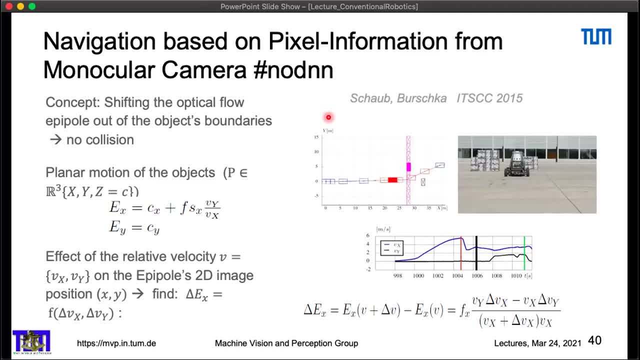 And it's writing the protocol for them. So understand dynamics. for me, It's now the current challenge And how to sync what you see with procedural description, So you may have a description of how to do something And now you want to see basically. 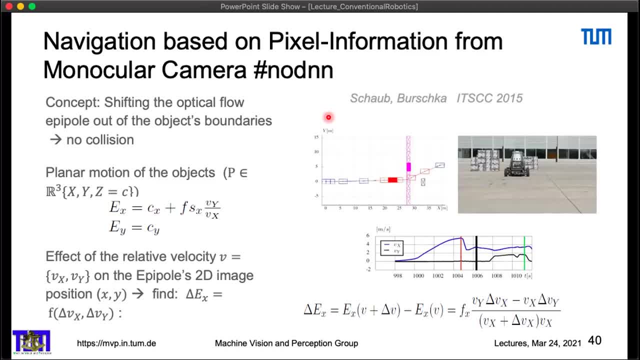 what you know about the process is actually happening in the front of you, or if you need to help, maybe because something is going wrong. Thank you, Any other questions? You know I'm happy to hear that I am wrong. I would really like to discuss. 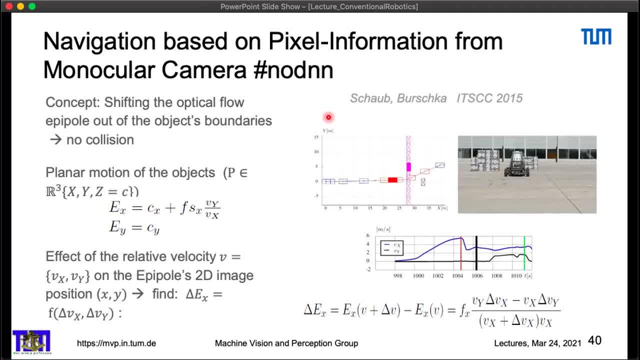 I kind of have a philosophical question, maybe about the husky versus the wolf thing. I was kind of wondering, maybe, that if, like, I was wondering if you think that that's like actually a smart system or if it's like a dumb system and whether, like a human, you 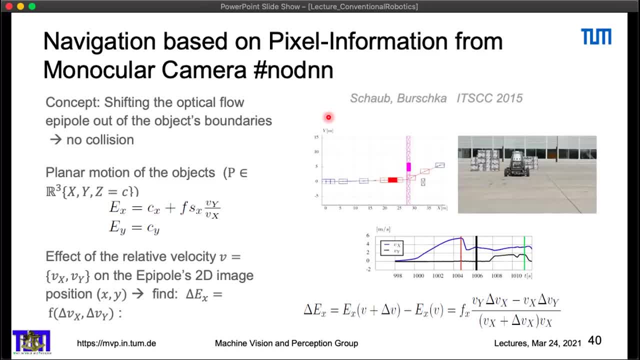 know like a human might learn the same thing from those pictures, And so maybe it's more of like an alignment problem where, like, we have something that we want to learn, but we're like giving it the wrong things to learn that thing. You just said the correct words. 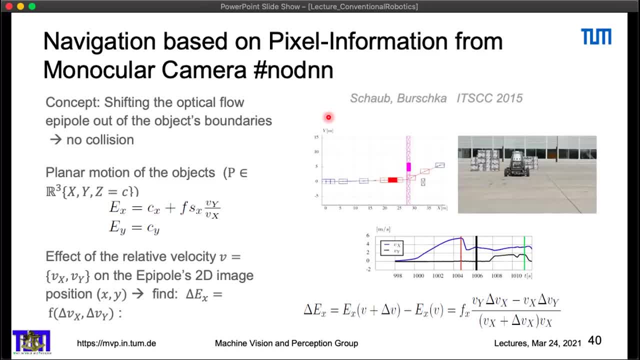 You've given the system the wrong thing And you haven't noticed. So I'm not saying that the system is wrong. In this case, the training set was wrong And whoever trained the system didn't even know. So my point is not throw away what you have. 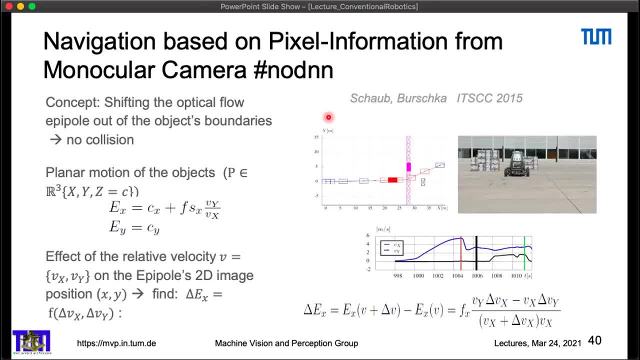 but try to understand basically what you're doing, Because in many cases people throw a lot of data at the network without really verifying what they really learned in the end- And this is what I'm trying to actually tell people. Try to understand yourself. 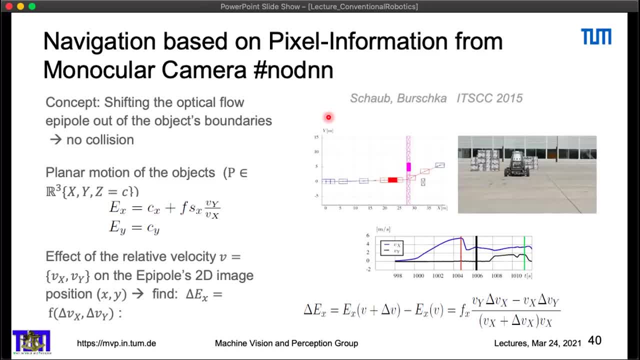 And for a robotic system to make decisions, you would like the network also to provide some information how certain it is. It's absolutely no problem to say I don't know, Then I would stop the robot. If you always say it's a bird and it's not. 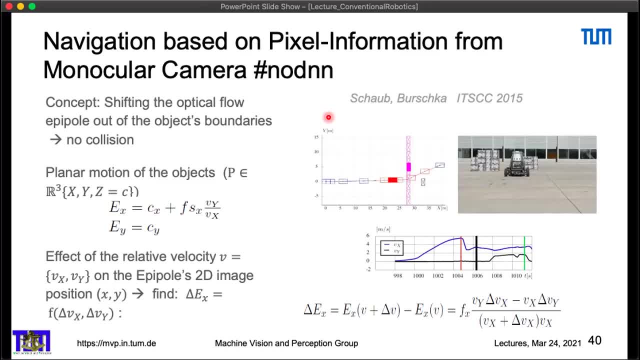 then I would do something wrong. So I was claiming at one point I had a big discussion with many people online And maybe you have seen it. I would prefer often a 60% accurate conventional system on the robot, which stops when it doesn't know what it's. 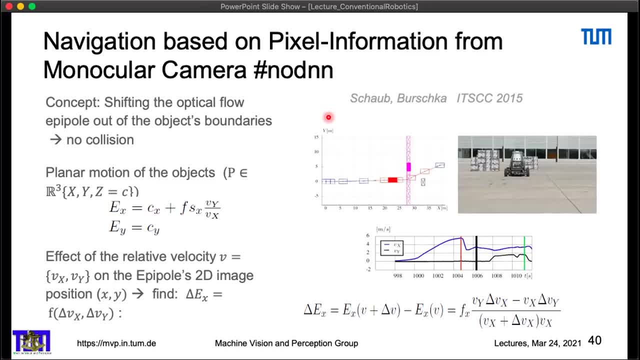 doing than a 95% deep learning system which goes 70 times to two minutes a day, nuts. So you're right. Yeah, it seems like that makes sense. It seems like it's possible to build a deep learning system that has that built into it. 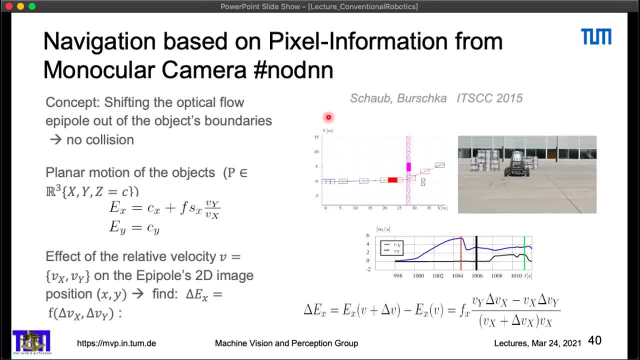 You know, the only people who actually have the correct data for it are these big companies, Because you as a lab don't have a chance to get the variety of data you need to train the network. So you get the robot system if you're Google or Amazon. 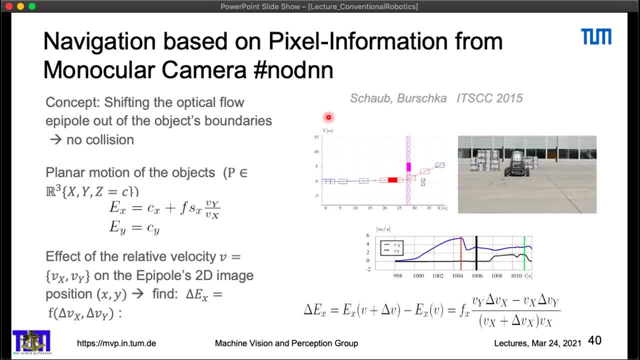 And you can train on the holiday pictures from all the people who use your account. But you will never be able to collect this data in your lab And if you do, there may be something which all the pictures have in common where the system will pick a cue. 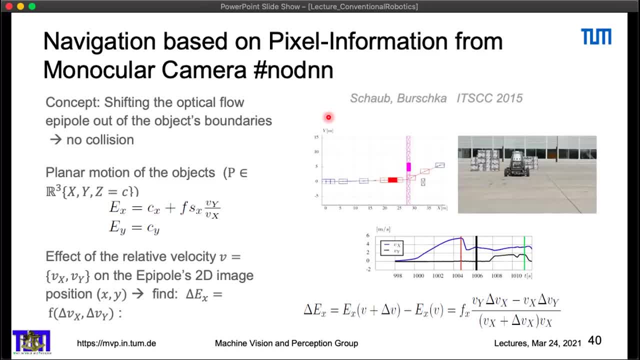 And then this is where your transfer knowledge doesn't work, Because now you put in a new environment and this chair the system was using for all the decisions is gone. Yeah, I wonder if that's related to, like, how we're collecting data and whether a robot working. 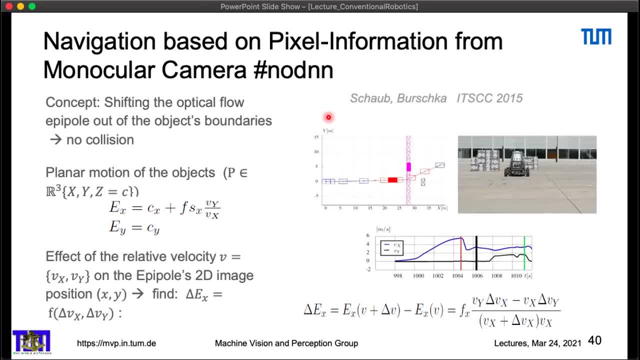 in the real environment would be better. I think I would really suggest that you understand the principles of what you're learning, even if you don't apply them, but understand what you're solving. And the second thing is you could learn a lot from 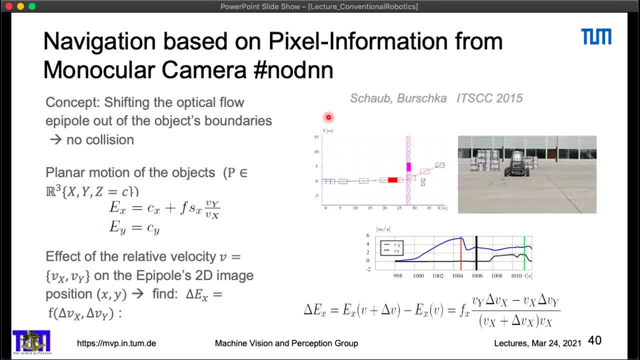 for example, people in the physics. They spent a lot of time how to set up an experiment. This is really a huge amount of work they spent to at least set up an experiment, And the same thing should also apply to deep learning. 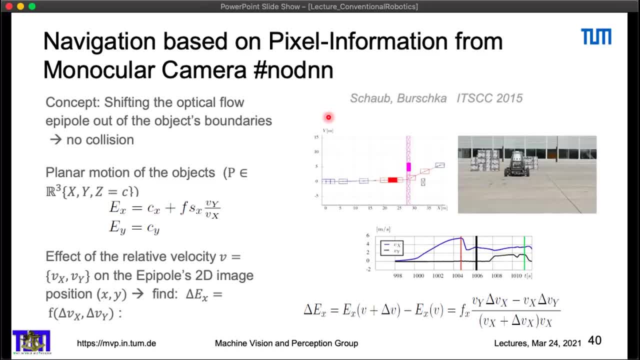 You should really make sure that your data does not have these wrong cues like the snow. OK, It's easier said than done. I know, Matt, you have a question. I can think of one. Just give me a minute. If someone else has one, then go ahead. 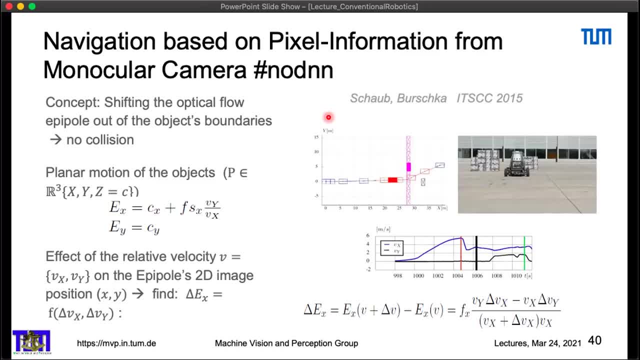 I just saw you turned on your camera so I thought you were getting ready to say something. Yeah, yeah, I was afraid that would be the impression. Darius, we have not yet got to neural networks And we will spend a couple of weeks on that. 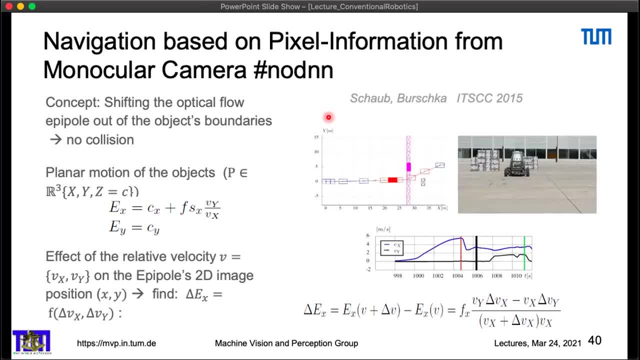 But I know that one of the things that is my goal is exactly for students to leave with. this is, if you're trying to use neural nets, make sure you check your data set, Make sure that you know what it's good for. 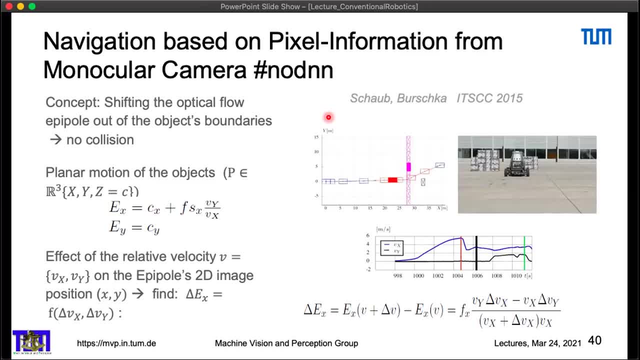 and what it's useful for. And there are a lot of data sets that are used everywhere- benchmarks and whatever- But what if you're trying to detect something? What if your new data you want to use has a whole bunch of things that don't exist? 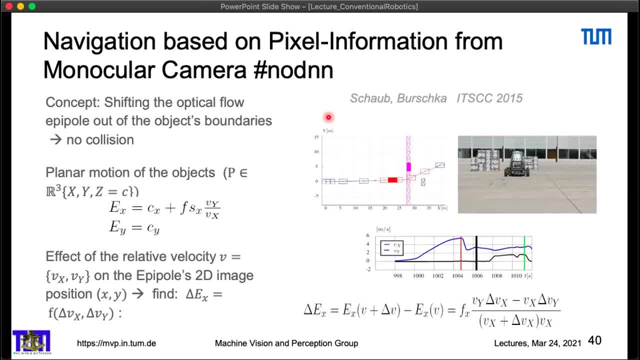 Maybe, Maybe in the data set that you use for training, Or the other way around. The training set has a bunch of things that it learned from and your environment doesn't have any- I don't know- chairs or something like that. 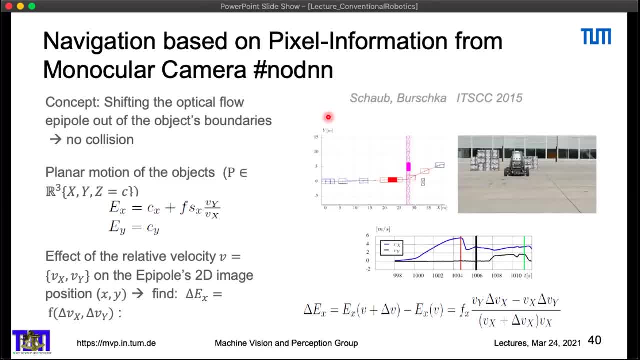 So then everything in the data set is going to influence. I remember Darius and I used to say that it's glorified pattern recognition. That's basically what the network is doing, And I know that paper that showed the visualization is like: which filter? basically which features? 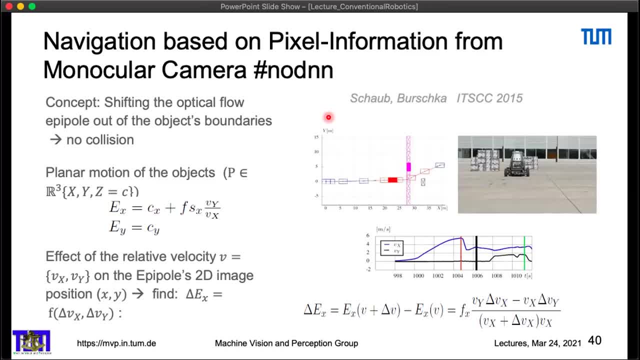 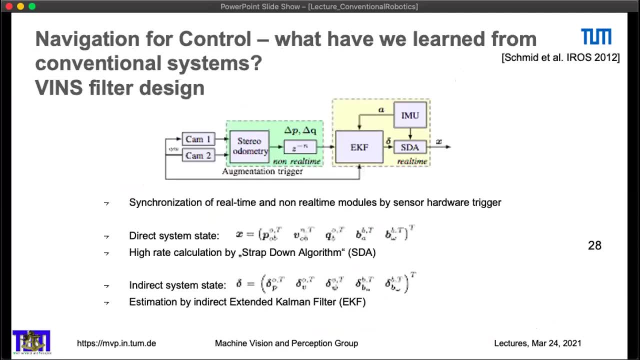 it's trying to pull in the first layer, in the second layer, in the third layer. That seems very intuitive. Oh, first we detect edges, then we put edges together and we detect certain orientation corners, Then we put this together and we found the spokes of the wheel. 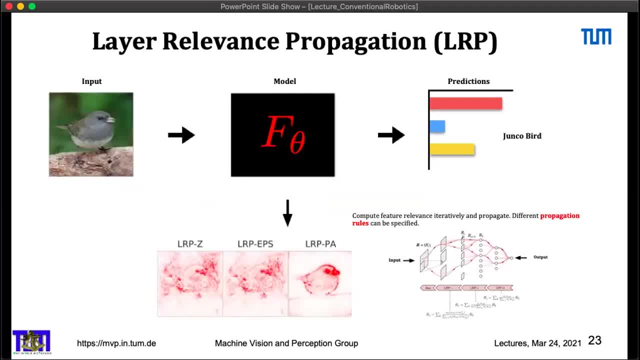 Right, If people would do this more, then we would learn more. Amazing, So you can learn more about how things work. I just put the slide with the bird. You see, doing this layer: relevance, propagation. you can see what different methods actually use. 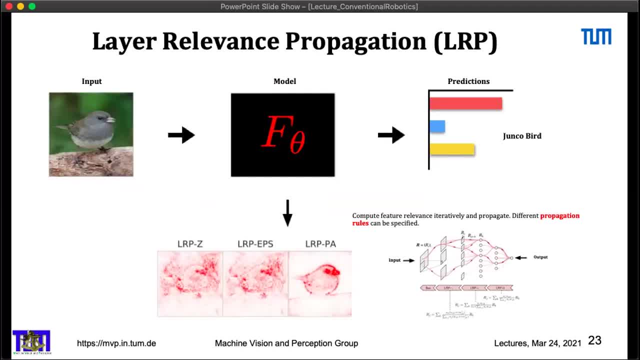 which pixels from the bird are actually used for making the decision. this is a bird, So this one is really focusing on the bit here. I think what you're saying is what I was trying to say as well. I would really like people to understand what they are. 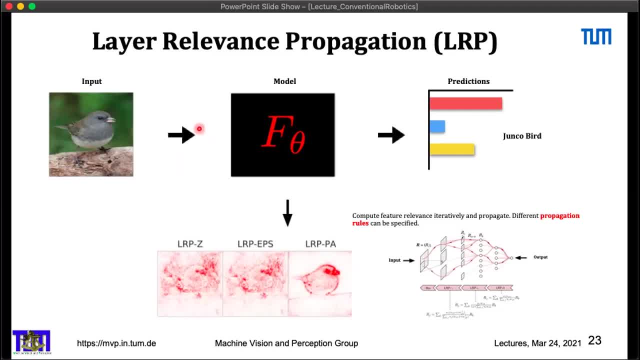 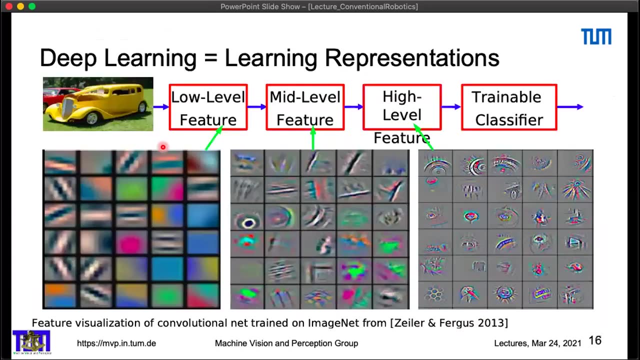 solving The problem is, of course, people who were developing the networks came still from the times when people were using- let's call it- conventional methods, So they were looking at the networks and tried to understand that there is these low feature extraction layer on the left. 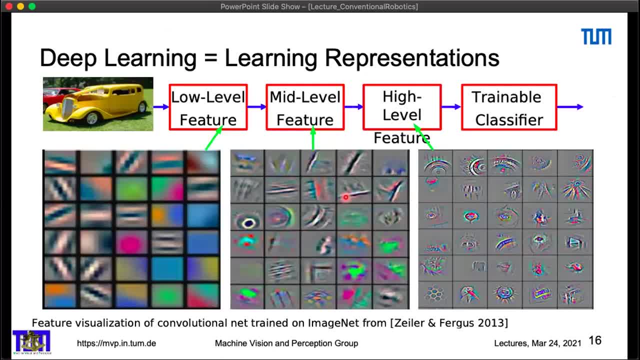 There is the mid features combining grouping. But what I see now more and more that many students are not trying to understand anymore what's happening, And this is, I think, a very dangerous thing, because you may train the network in the wrong way. 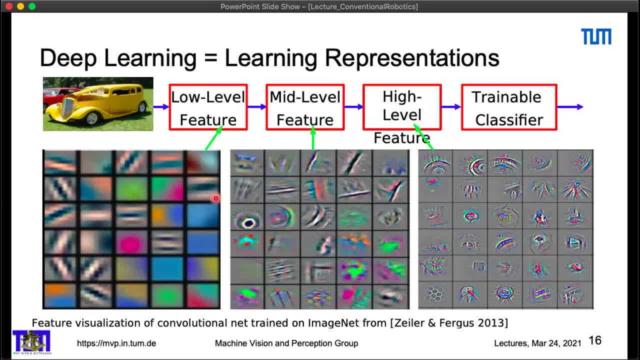 If you don't understand the underlying problem, you may make mistakes in your training. So I'm not saying don't train, but understand what you're doing. You want to be, You want to ask more from us, from your teachers, who are teaching you things right. 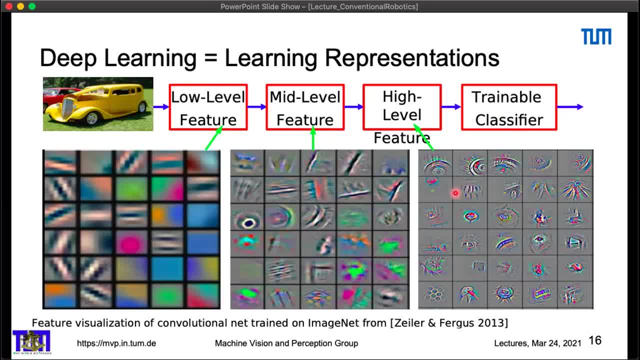 You. So you understand. Yeah, A lot of students can graduate and just go through a few tutorials on TensorFlow and do a few projects And they feel like, wow, they've done so much stuff. right, There is room, There are jobs in the industry that care about this. 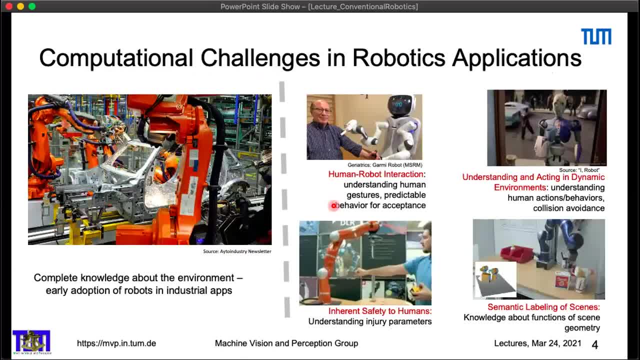 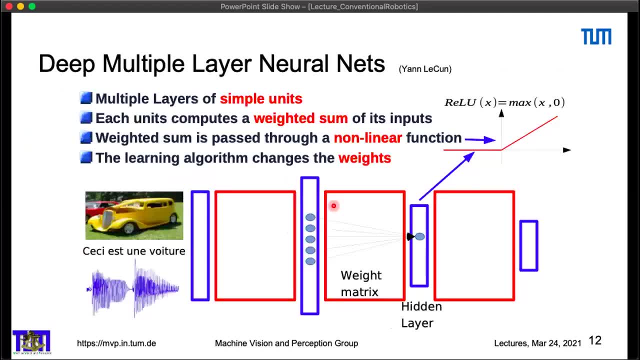 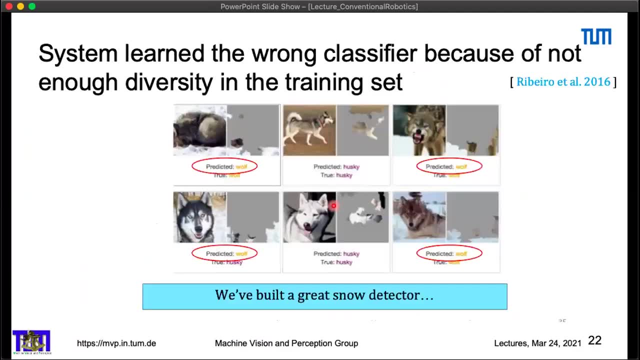 And actually I have a friend who works at Facebook. He's been there for a really long time, But they were saying that they're trying to apply Neuronets and deep learning and their goal is to basically derive more advertising, more advertising. 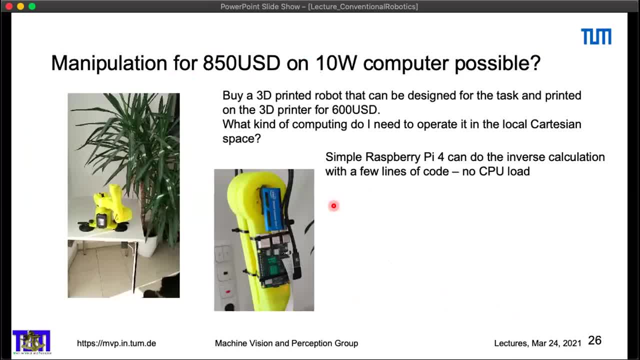 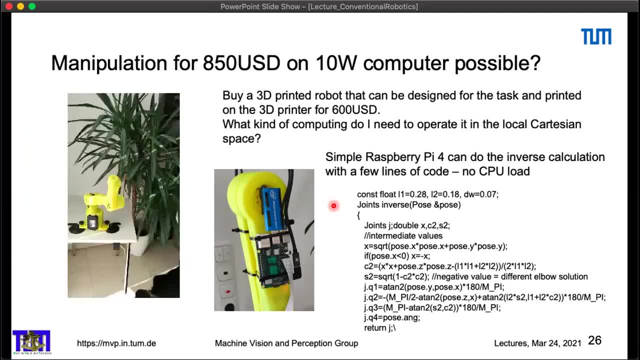 money right, And he's saying: I am willing to hire the smartest students that are out there and pay them a lot of money because if we come up with an algorithm that improves by a quarter of a percent, that will pay everyone's. 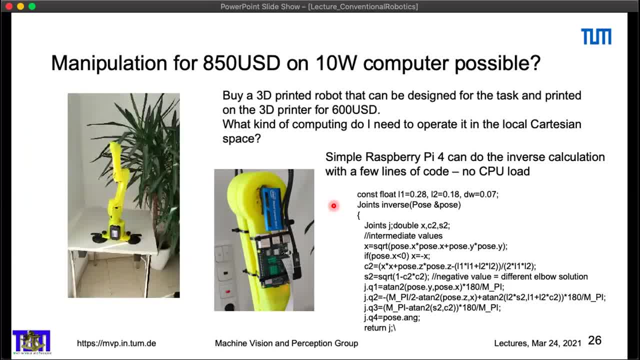 salaries And Facebook will be super happy. But to get that extra quarter of a percent you really need to dive deeper. You can't just push train and push play and say, woohoo, look at my beautiful result. You know. 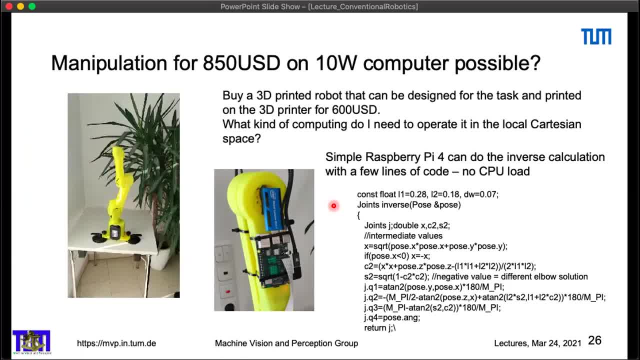 Just to motivate also the students a little bit more. I have now multiple projects. Actually, I have a company which is working now on- you would be surprised- train localization. I was smiling before. Why do you need to localize a train? 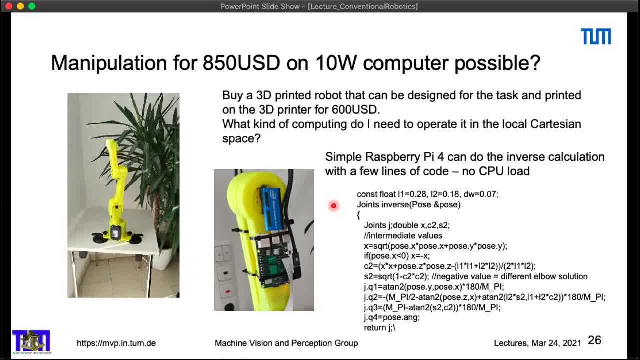 It's always on the tracks. It's an important thing To understand physically if the train is still all together or if it lost cars, whatever. And to do this you cannot apply deep learning at all. I had to modify my conventional vision system. 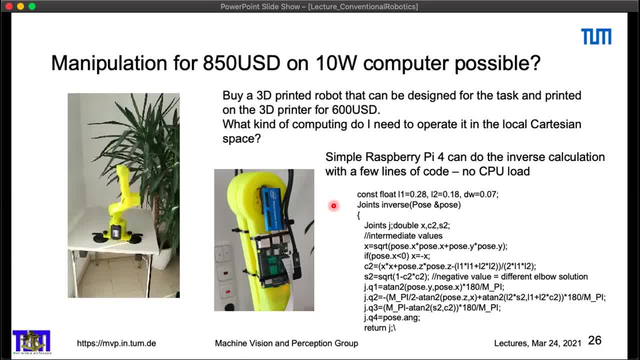 to remove all random number generators from my system, So I couldn't even use RANSAC. Why They need certifiable systems. To have a certifiable system, if you apply it to an image, it needs to give always the same answer. 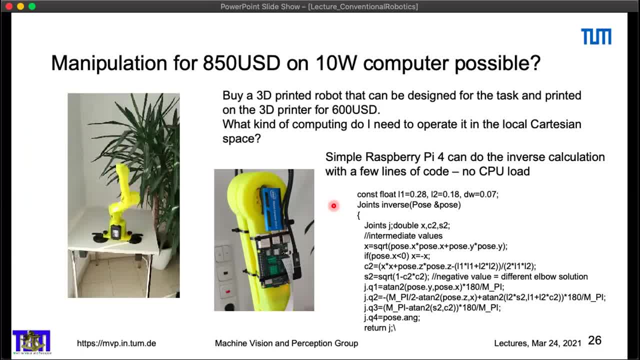 And this is something which cannot be done for now with deep learning, And the same is true. I'm always surprised how much people trust the Tesla autopilot. I would be scared sitting there And I would feel a lot safer if the pilot would tell me. 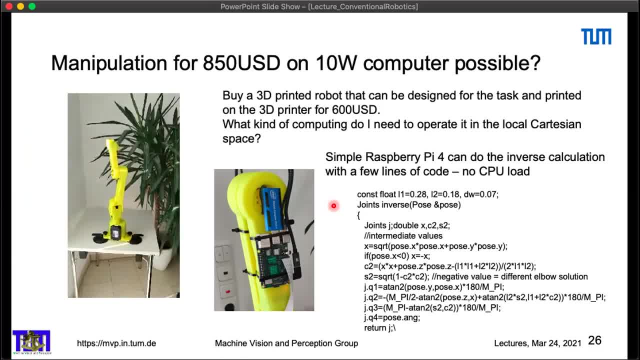 its confidence value so I actually can prepare to catch the steering wheel if something goes wrong. Like you know, I'm completely fine, The system telling me this environment is not too familiar for me and not just claiming I know what I'm doing. 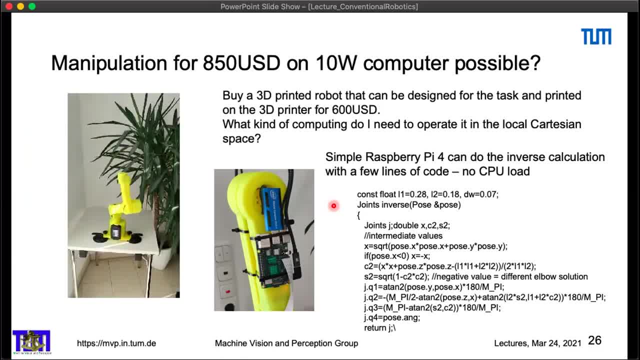 I'm going for it. So I think we hold, Sometimes I think we hold- robots to a higher standard than humans, though, Like often, I don't think humans do that very well. A lot of the videos I see from the Tesla drivers kind of sleeping in the car. 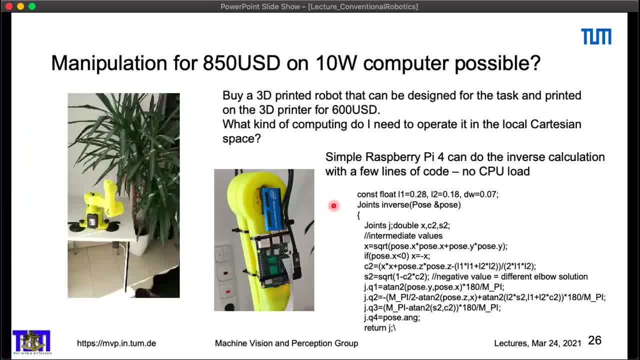 of course are people who have no clue what is actually working there, So they have too much trust in the system. There's a lot of wishful thinking. I think they should also do better on message and say: you know, this system would be better for trucks on the highway. 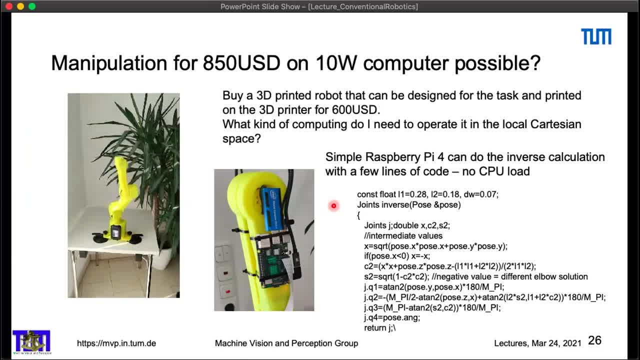 but don't try it anywhere else. When I was doing my PhD in the 90s, there was a professor in Munich, Dick, who actually was driving on a highway up to almost 150 kilometers an hour with a transputer. 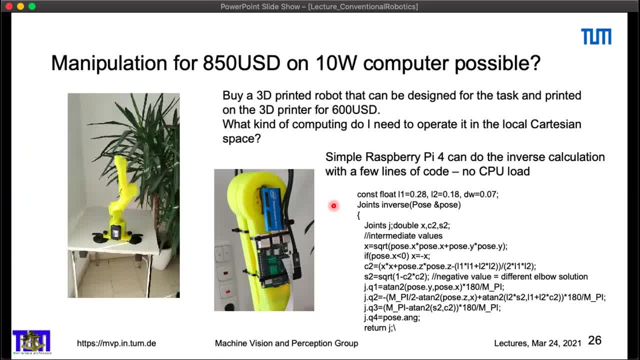 I think you guys don't even know what a transputer is anymore. It was a specialized computer to do image processing, because back then the CPU power was what your current keyboard is doing, And he was driving 160 kilometers an hour on the highway with this. 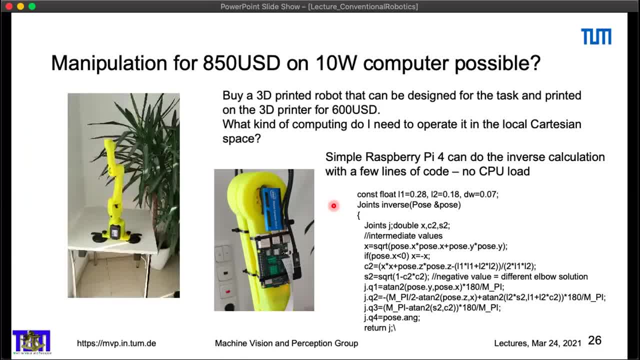 And then people were asking him once why he's not driving from the city And he was saying, well, it's very difficult, And you would be surprised how often your Tesla autopilot is just guessing. You just don't see that. you were just lucky getting through the scene. 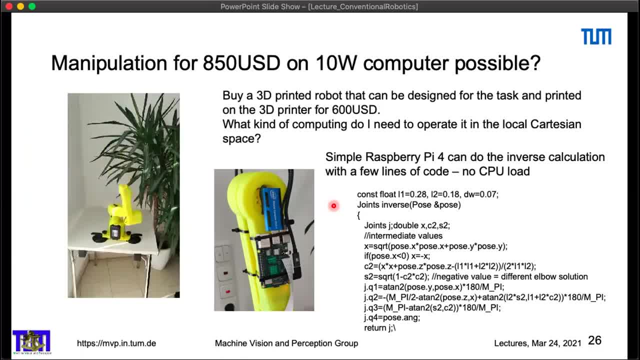 Just an 80 percent of what you see on the road can also be solved with very simple Lane following and things like this. The problem is always the challenge in this exceptional situations, And that's where you would like to know if the system is still doing fine or not. 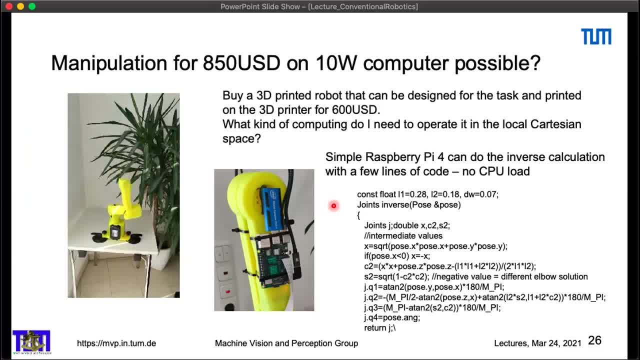 Driving on an empty highway. I trust everyone that can do it. You just follow the line. But I see more and many of my friends- I have many friends. We have in Munich, many companies here. So many of my friends complain that they cannot find people who are really 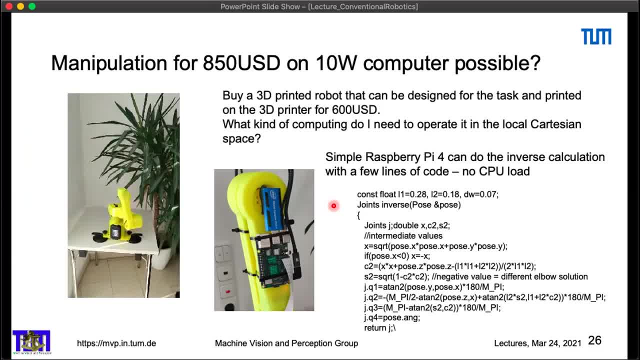 really still can, for example, apply a common filter, For example. we're going to talk about that next week- How to how to fuse information- But I got mad at my student. My class is usually 400 students, so it's always entertaining to teach. 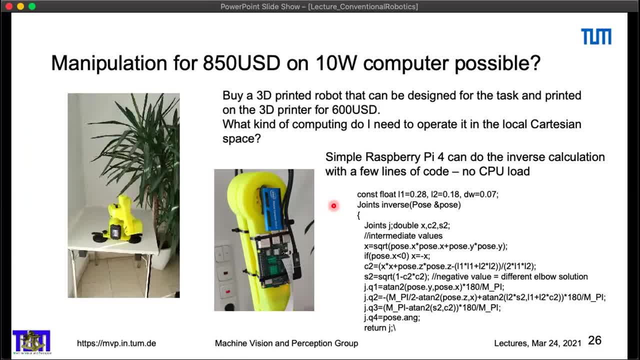 It's like in the soccer field, But I had all of the students like I finished common filter And then the student came to me like why do I teach it? You can learn it. You can imagine I was very happy about this question. 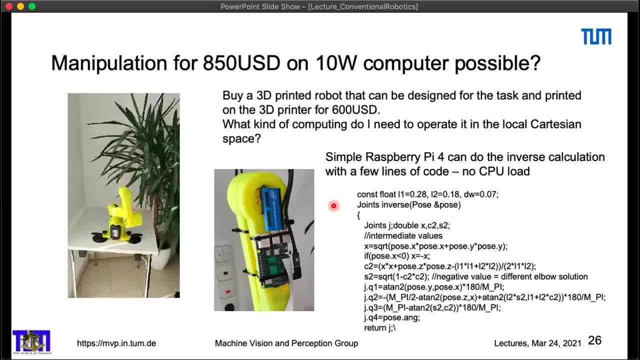 Yeah, but you know, I think, if there is an analytical solution, why don't apply it? This is why I took this example here. Like I don't need to learn inverse kinematics of the robot, This is known to man: how to calculate. 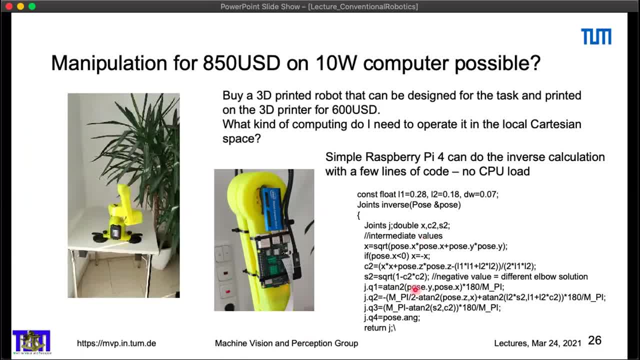 Why don't you use it? I still, and I even know how to dynamically improve the parameters, how to actually learn the learn in the old style context or adapt the parameters based on my- my errors I've done during manipulation. There is where we're getting close to the end of our time. 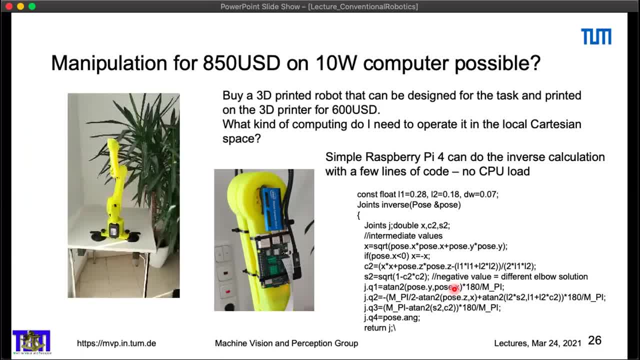 Does anybody have any other question? Yeah, I actually do have a question now. So you were talking about with. so I don't really know machine learning too well, Like I'm a mechanical engineer actually, so I'm not too familiar with a lot of computer science practices. 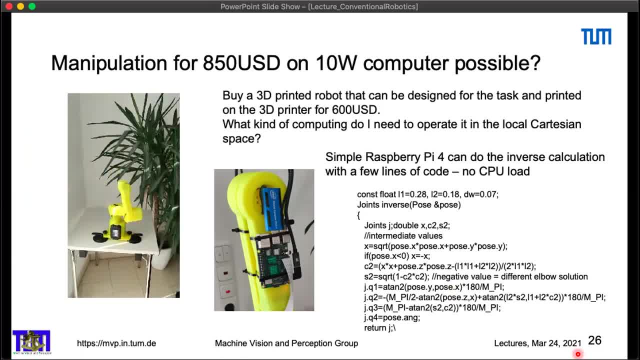 So forgive me if I am a mechanical engineer too. So, like in machine learning, like you're saying, like only these, like big companies, have access to these, like large data sets, like Yeah, so like, how do you eventually reach a point where, like you can have enough data? and like getting more data points and getting more images? 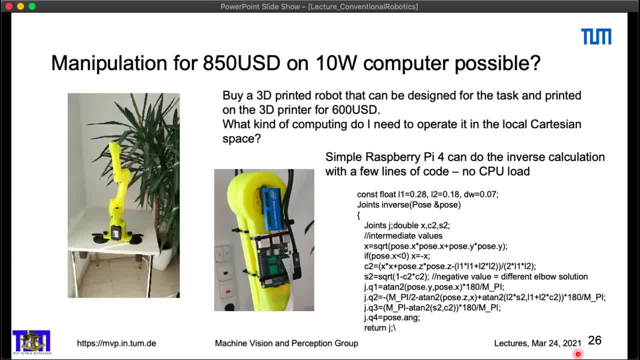 whatever like isn't really going to improve, like the model and like how I mean. I guess that would depend on the application. But like you know, I'm not sure if you would be talking about this- But of course the big problem always with all these learning approaches is overfitting too much data that the system starts kind of to 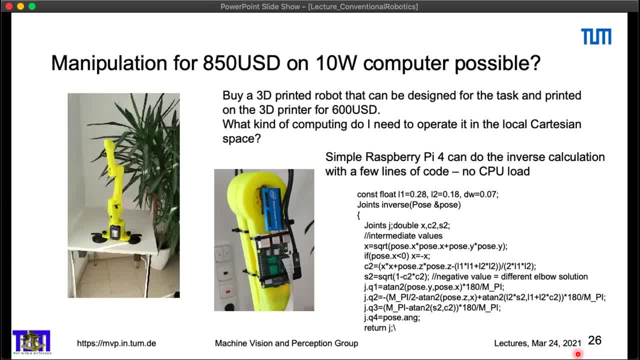 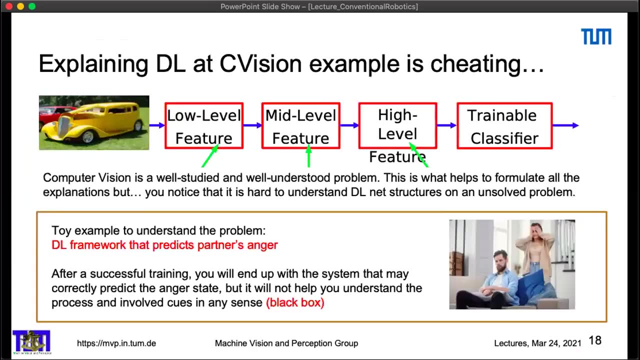 You could think about it's rebuilding a really complex separation function which is not really necessary now. So you know, the important thing, I think, is what I was trying to have on This slide here is basically to understand what the learning is doing. 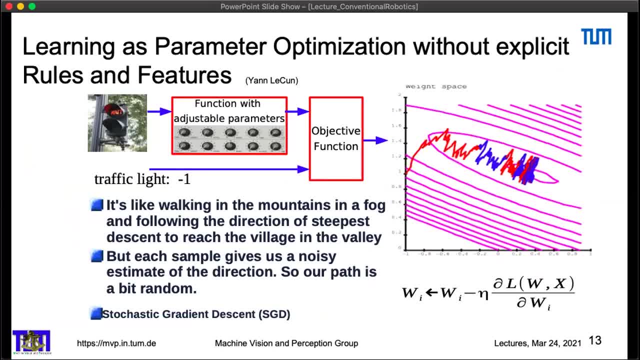 You spent a lot of time now repeating the learning just because you have very small steps in the gradient descent. So, like gradient descent, if you do optimizations, like the worst thing you can do, and this is what the whole system relies on In optimization, in the regular optimization. there are many other techniques that are better, but they require, of course, some underlying model to run. 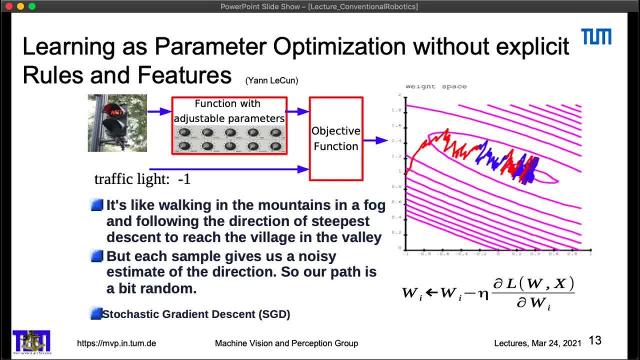 If you don't have a model, You do the simplest thing, and this is gradient descent, And that's what the whole learning approach is based on. But I am reading, Darius, that you know I see things at conferences too. 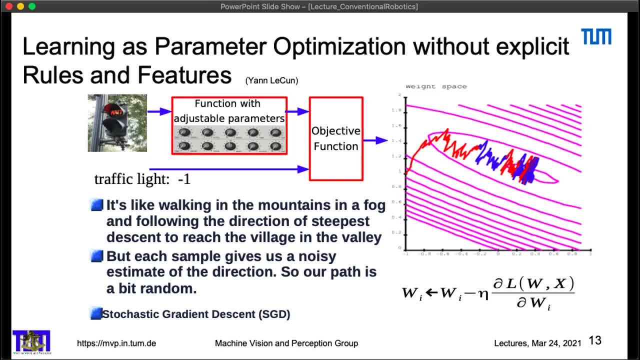 People are starting to try to bring more information about the model into the network from the beginning Right, So I know that more and more people are aware of this. For learning. it would be nice if, let's say, you train the system. 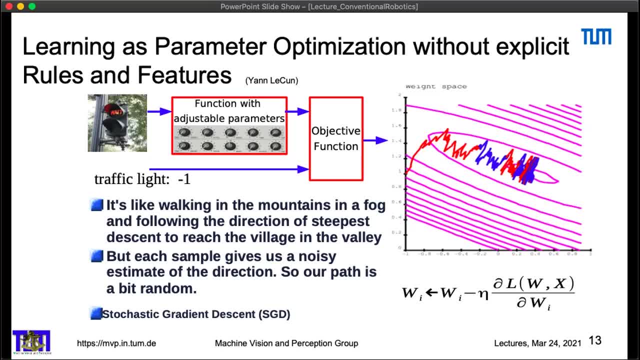 I was making one because recently There was this announcement that Google trained one trillion parameter language model, or something like this, And I was saying like, OK, let's invent a new sentence, Then they will have to train it from scratch, because the current system require you to train all the data again. 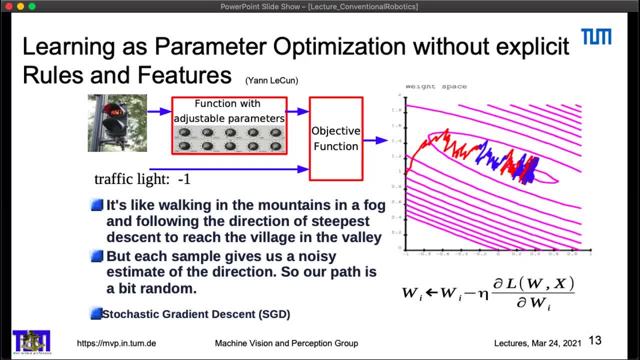 You cannot incrementally. Yeah, that's another thing that's not accessible to the incremental knowledge acquisition which humans are doing all the time. It's not really working yet. So I think, instead of inventing another application, The application will make more sense. to try to understand what I like the system. 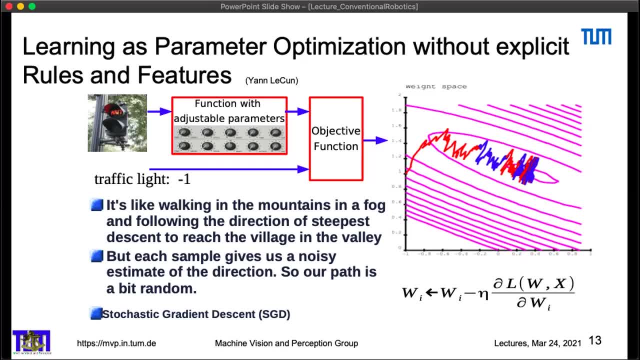 I just don't like the way it's used. There is a question in the chat from Gerhard: What got you into computer vision and what? what got you into computer vision in the first place? I was working in the lab and the job I got was predict laser information- the 80s- and I got interested. 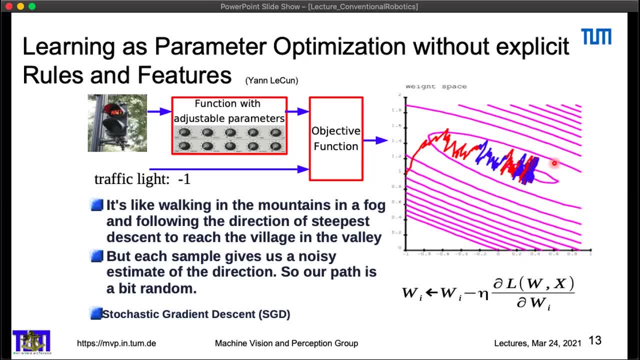 Actually, originally I wanted to be to become a cameraman. I kind of became it now in a different context. I like to understand basically the perception, So this is also what I skipped it completely. I really like how to combine perception with execution without going through 3D representation, because I think humans are not, for example, working in 3D. 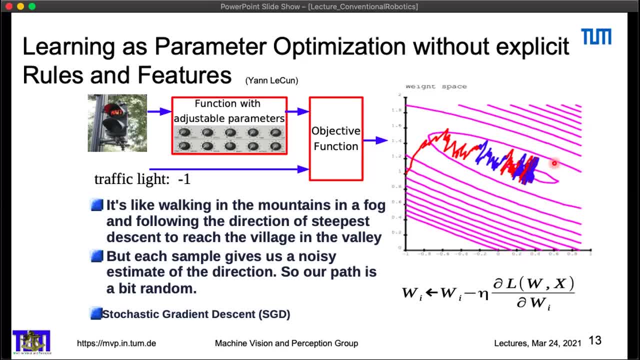 But depending on the task, they have some representation. they validate with the vision And, like the typical example, if you do Robotics maybe the person from mechanical engineering will know it is visual servoing. You can really map the visual input to some output space using a Jacobian. 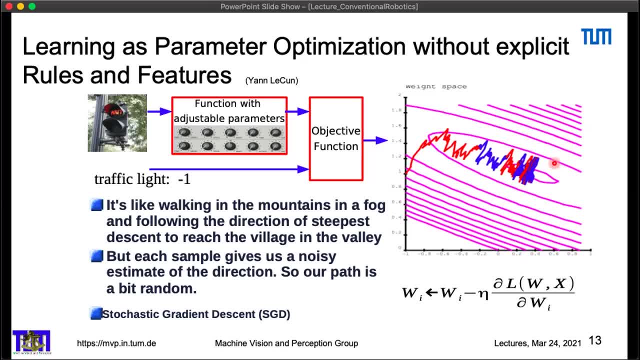 Which can avoid completely going through the 3D space, And this makes things more robust, and something like this interests me, so I really like to work with perception models, And this is what got me there. Darius, I have a cliche question. 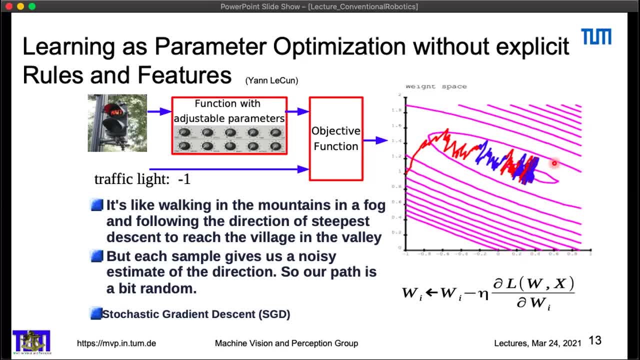 I mean a cliche concept here. Is it that in Germany, I mean, if you're in an engineering school, there's just robotics everywhere, so that you know, people are more likely to, like you know, turn to studying robotic systems and 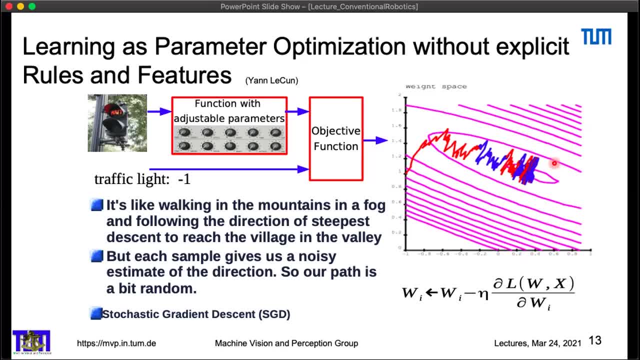 Because here in the US, especially as I'm trying to find things for my kids to see, I find that that's not so easy to like go to even, you know, a summer camp or some sort of expo where my kids can play. 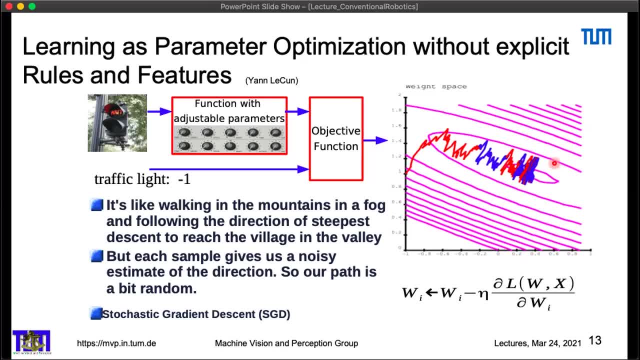 You know right, They're robots. You know we organize. actually, there is a robotics fair called Automatica, which will happen for this year. Munich is an exceptional place with a lot of companies and startups, So if you talk to someone from Karlsruhe, you will hear a completely different story, I think. 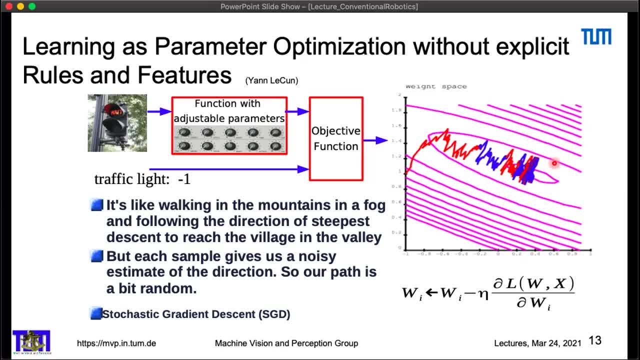 So we have here the Munich School of Robotics I am a member of, And we have Siemens, We have Google, We have Apple, We have SAP, We have Google, We have Brain Lab. We have tons of companies around And, of course, we have BMW MAN. 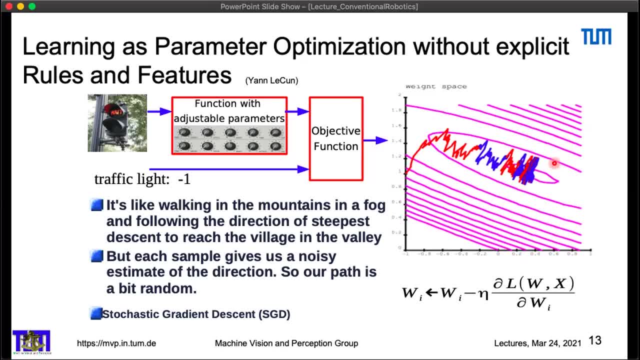 So we have a lot of companies around us, which actually motivates a little bit more. So that's why, also, we are more interested in system applications of what we're doing. We are not really doing the job for Google or Amazon to collect data and label it. 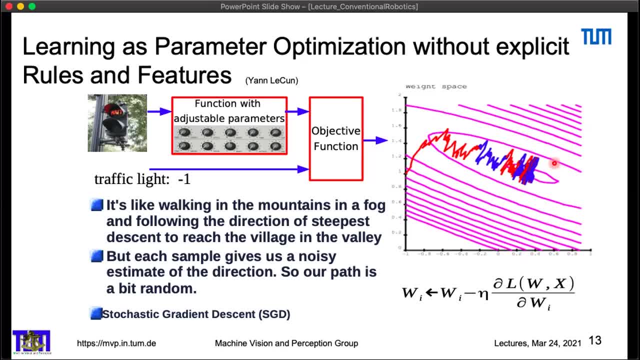 They are more interested in how to control something. This maybe explain also why I'm looking at it from a slightly different side than the whole thing. Yeah, definitely We have lots of people doing like Daniel Kramer's pure deep learning vision. 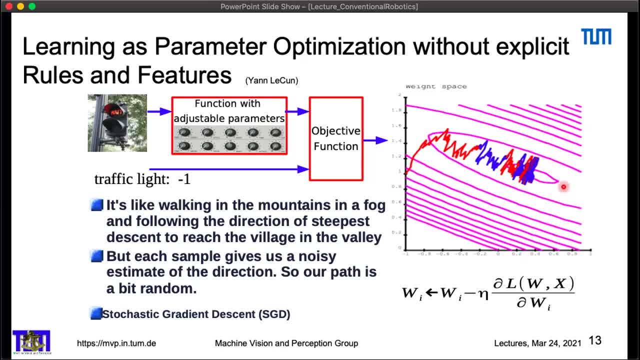 And just don't get me wrong. I was doing neural networks in the 80s But my old advisor got it out of me because I always tried to sell a system to him and he was always asking me for proof that it works. 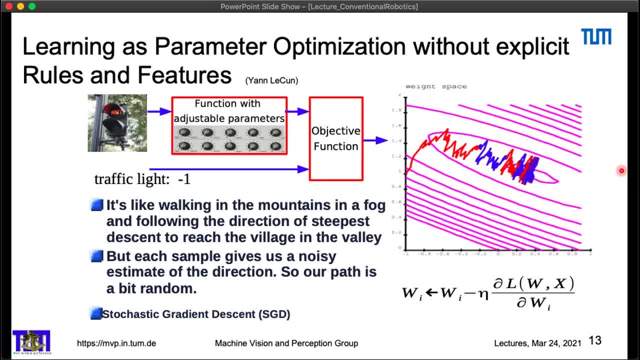 And I could never prove it. I was doing neuro-fuzzy. I'm not sure If you do know fuzzy logic still, but I was trying to do neuro-fuzzy, kind of combination of fuzzy logic which is kind of similar to what you're doing now. 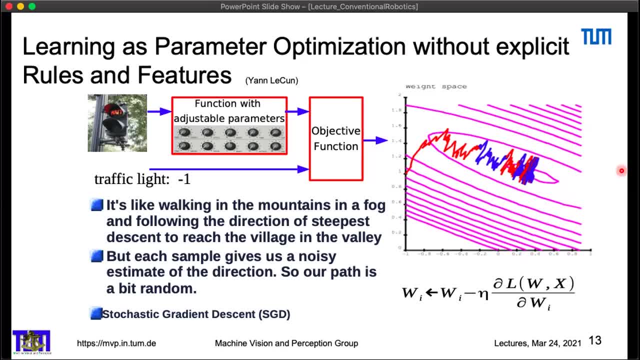 Gone. Thank you so much. I think the students are going to be heading to another class soon, very, very soon. Guys, I'll let you know about Friday. Like I said, I'm leaning right now on taking the day off.